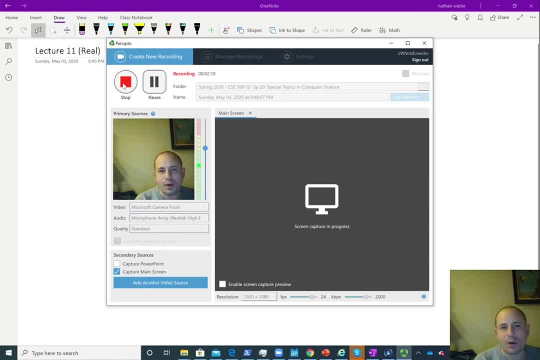 in this course, such as with quantum. you, whenever you measure the system, you run the risk of damaging it. So detecting the presence of errors is a lot more subtle with a quantum computation than it is with a classical computation. The next issue is that, of course, 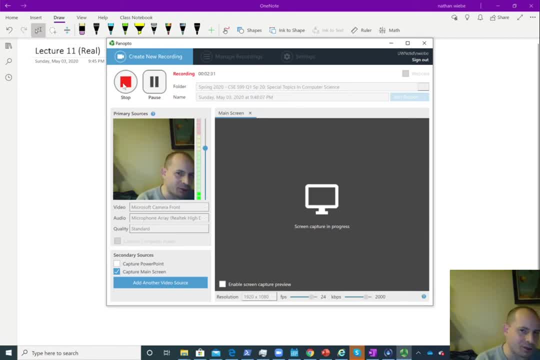 there's a no-cloning theorem. Well, there is as well for classical probability distributions, but that being said, that does prevent us from just abjectly cloning a quantum state and using this to create redundancy for our programs. And finally, the other thing. 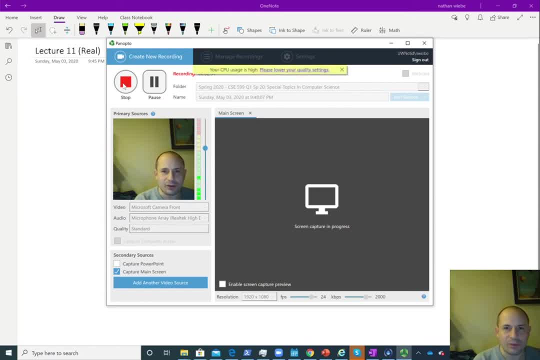 is that errors in quantum are continuous. You could have an arbitrary unitary describing your error. In fact, you could have something which you could view as a probabilistic mixture of unitaries affecting your quantum computer, And that is very different from the bit flip model. 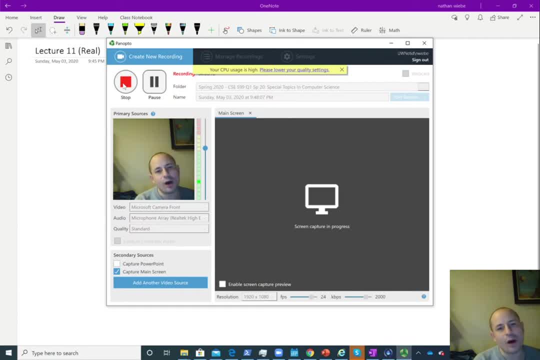 that people normally consider in classical computing. So I'm gonna begin by first doing what I usually do when it comes to these topics is I'll begin by talking a little bit about the classical version of error correction, And then what I'm going to do. 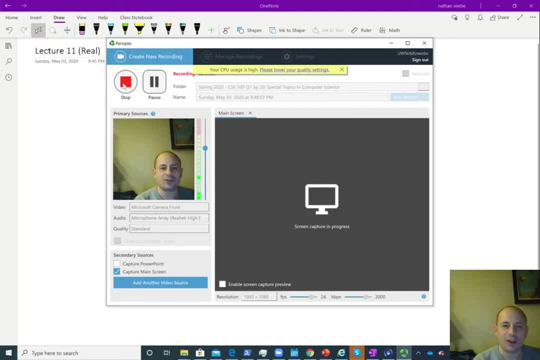 is I'm going to begin generalizing this and talk about how we can do error correction in a quantum setting. So today, what I'm going to be doing is I'm just going to be talking about building up the showing how to resist bit flip errors in a quantum computer. 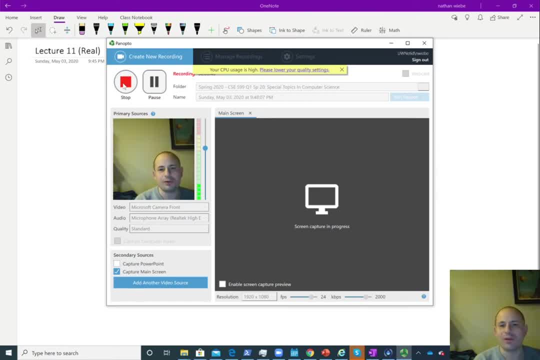 by encoding your quantum information in sort of a degenerate subspace of a higher dimensional system. And then what we're going to do from there is next lecture. we're going to talk about how we can make this resilient also to fit random phase flip errors. 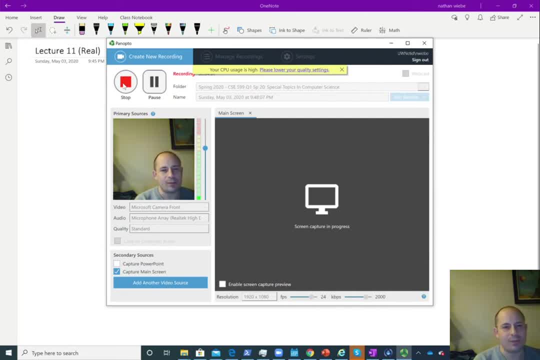 and argue that once we have a code that can detect and correct both bit and phase flip errors, that actually it will be capable of correcting every error. Now, this is a totally unobvious fact, but it's key for for us in quantum error correction. 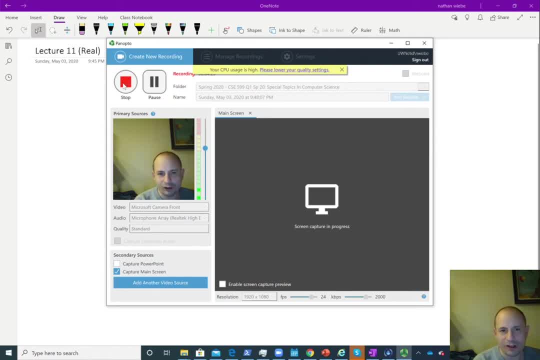 And the idea, basically, is that what quantum error correction does is through measuring auxiliary parts of the system. it's actually capable of projecting arbitrary errors down to discrete errors that can be corrected, And this is the thing that's magical about quantum computing when it comes to error correction is that 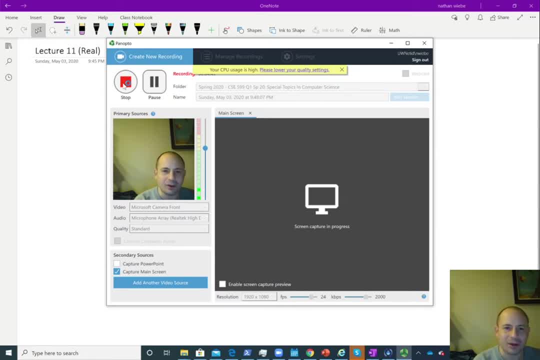 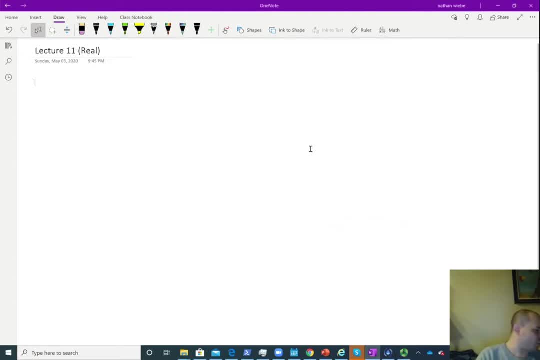 So let's begin by talking about the very, very first idea in classical error correction, which is one that you probably are already familiar with, but that's why I'm going to begin with it And so simplest way that we can deal with this. 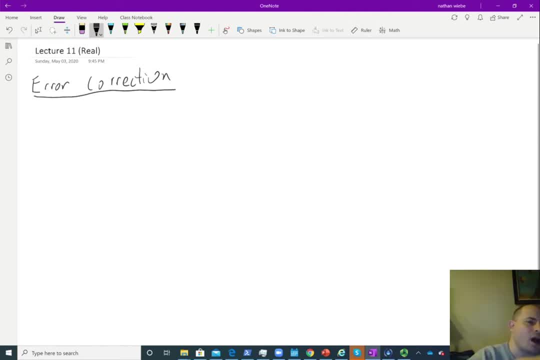 is kind of majority. it's majority voting, or the repetition code, as it's often called. So the idea of the repetition code is pretty easy. Imagine what we've got is we've got a bit right, So our bit value is either zero or one. 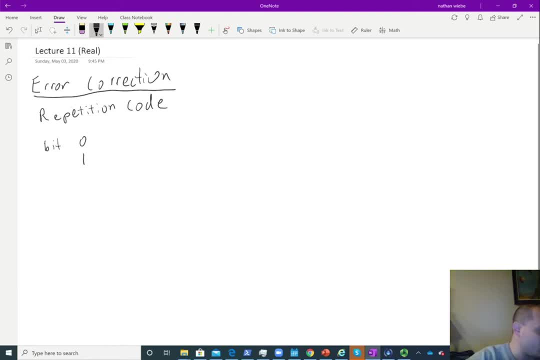 And now the way that we're going to envision modeling a noisy computation is that imagine, with probability p a bit flip occurs, That is, we end up getting x goes to not x for any variable x, And so this is what we're going to have. 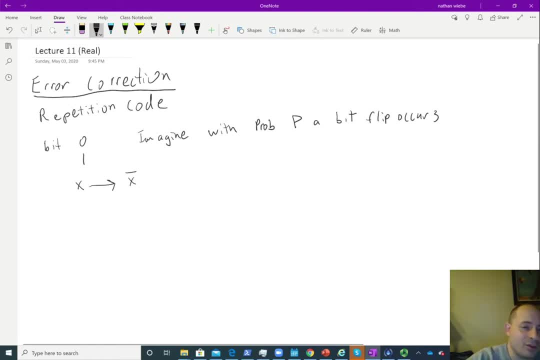 And we'd like to be able to build some redundancy into this. And so this is what we're going to have, And we'd like to be able to build some redundancy into this. And so this is what we're going to have, And we'd like to be able to build some redundancy into this. 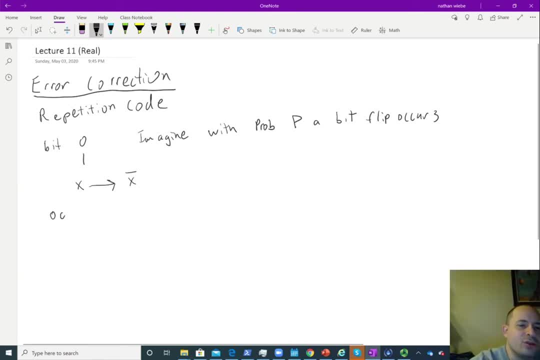 The simplest way to build redundancy is to do the following encoding. we will end up saying that we're going to encode 0 as three zeros and 1 as three ones and 1 as three ones. Okay, we'll see in a second why 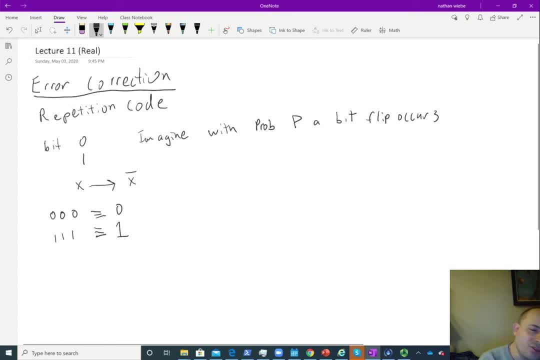 I pick 3 rather than 2.. Okay, we'll see in a second why I pick 3 rather than 2.. But this is the simplest sort of repetition code, And so the idea basically is the following: And so the idea basically is the following: 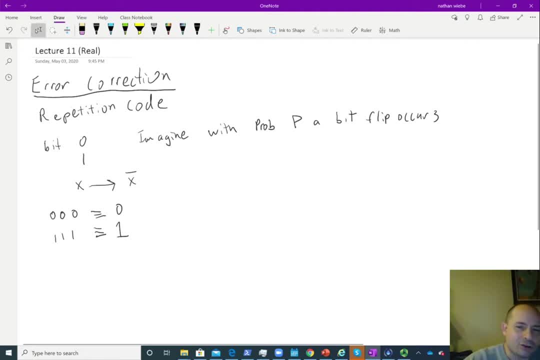 Let's envision that an error actually ends up happening. Well, the error- let's say this bit- ends up getting flipped randomly. That will end up causing this code word over here, 000, to go to 001.. Similarly, 111 will map to 110.. 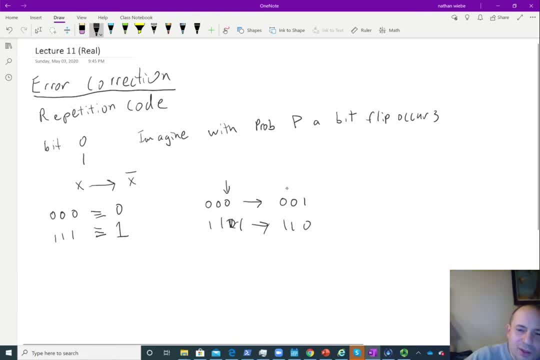 Now, by taking a look at the structure of this, we can see that there's two zeros and one one, So therefore, this is closer to the original code word that we had, versus this over here, which is closer to that one. Now, these two are completely distinguishable. 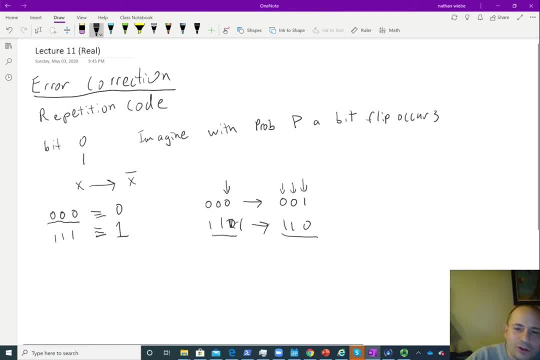 However, if we ended up having two bit flip errors, we could end up getting something like 00 goes to 011, which is actually closer to this over here. This would correspond to what we call a logical error, where the errors in the redundant encoding of the bit accumulate to the point where our decoding process 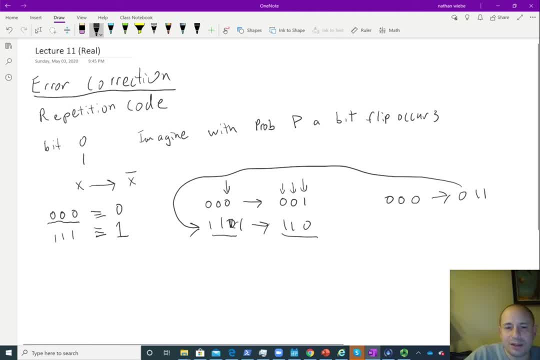 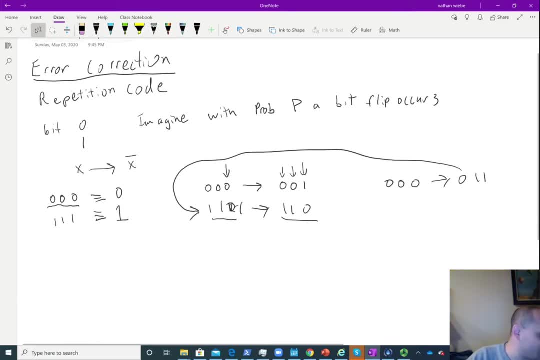 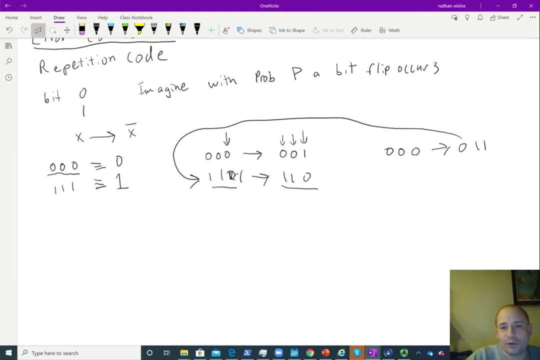 ends up saying that actually we're more likely to be the other bit string than the former one. So that's basically it, Thank you. That's basically the idea behind this. Now to see formally what we end up meaning by this, it's actually nice to think about this in terms of probability. 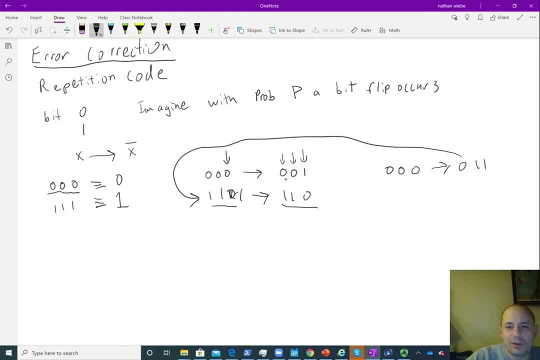 So we can think about this, say decoding the one bit flip case. So in the event that, let's say, we measure 001 coming out of the repetition code, Well, under this assumption, the probability that we end up getting this, 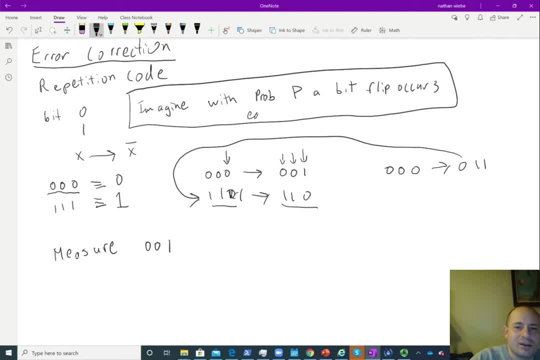 and assuming each bit is IID is independent and identically distributed. independent, okay, measure. okay, say we measure 001.. What we want to be able to do is we want to be able to compare the likelihood that this would end up coming up. 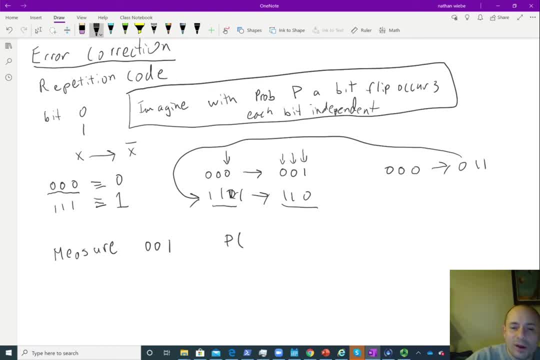 The probability in this model that we would generate 001, given that 000 is the true one- is equal to the probability that we don't flip on the first one times the probability that we don't flip on the second one times the probability that we flip on the third. 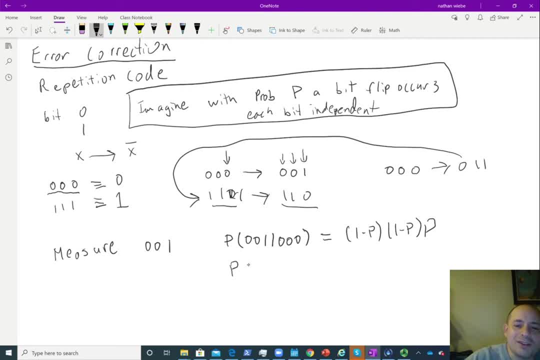 Conversely, the probability that we would have gotten the same thing, given that we have 111, or, sorry, probability of drawing 001,, given that the truth was 111, is equal to well. we need to flip now the first two bits. 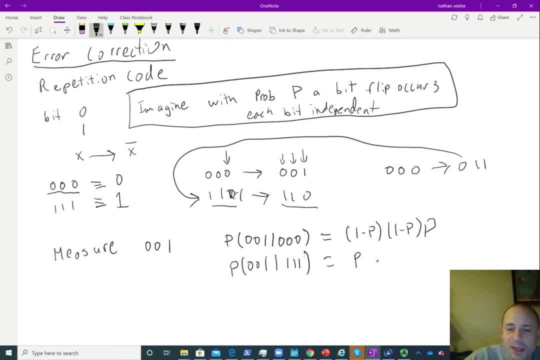 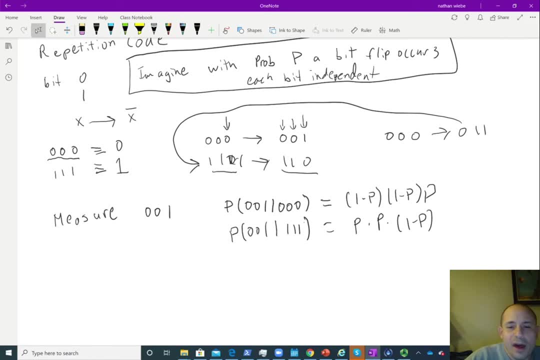 but leave the last one the same. So this would be p times p times one minus p. So you can see in this case that the likelihood ratios and the ratio of probability between all of these is actually just going to be one minus p over p. 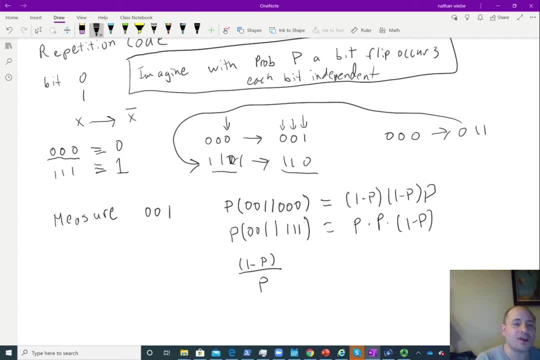 So in this particular case, let's consider comparing to the case where we just have the bare qubit. If we had the bare qubit or bare bit, we'd have zero and one. Now this is going to flip to one with probability p. 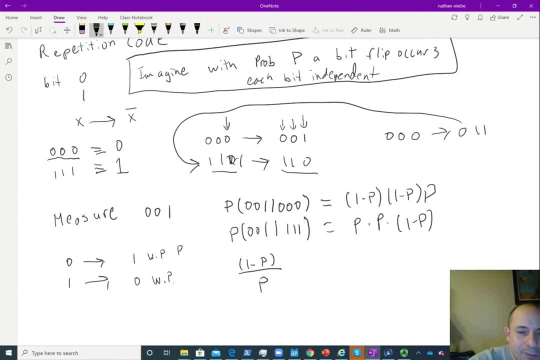 and this will flip to zero with probability p. So the probability of an error occurring over here is just simply p, And the likelihood ratio that we end up getting for this is going to be simply: yeah, okay, nevermind. So the point is: 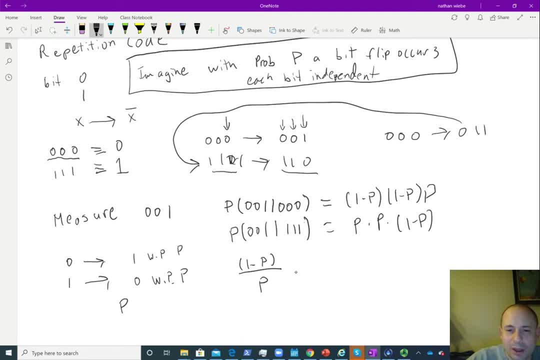 is that this likelihood ratio that we end up getting over here for p less than one half is greater than one, Meaning that in the event that p is some small value- like, let's say, that p was equal to 1%- then what we would have is we would have: 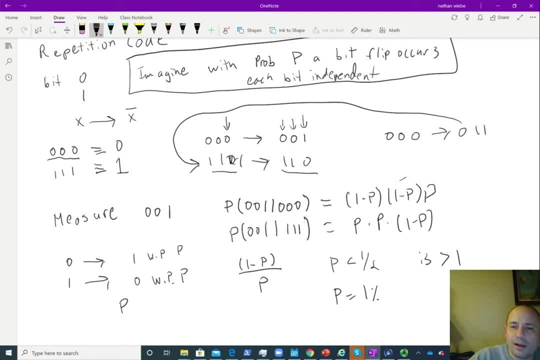 with overwhelming probability, this is the more likely model than that one, Meaning that it's much more likely that the data came from one error happening on 0, 0, 0 than one error happening on 1, 1, 1.. 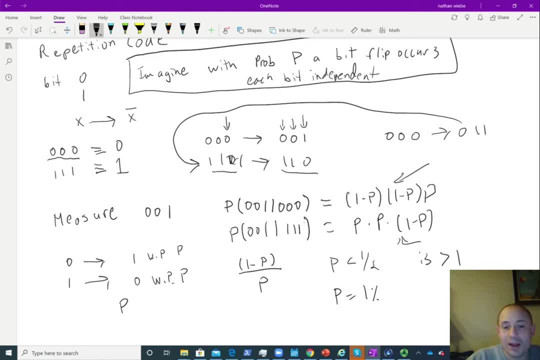 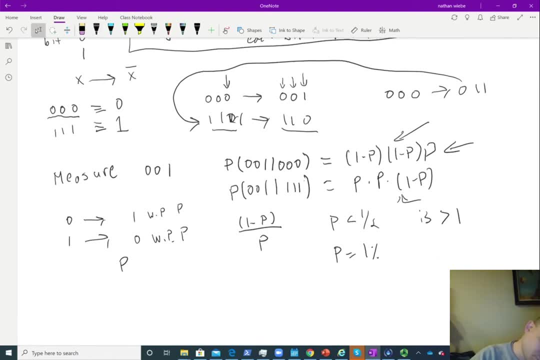 So that's how we end up doing it, And in the event that we decide that this is the correct course of action, then, based on this likelihood ratio, this likelihood ratio test, we say okay, the third bit is the most likely one to have flipped. 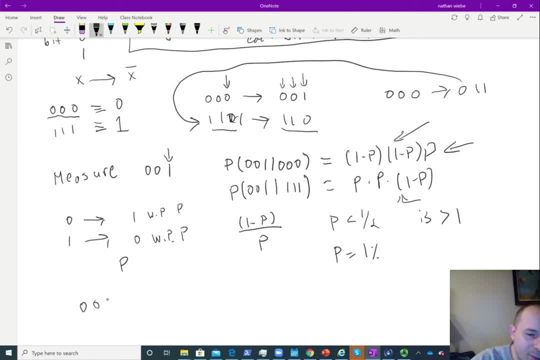 And therefore we can do a correction. We can just take the bit string and flip the third bit to end up getting 0, 0, 0 backup. So that's how this whole decoding process ends up working. But you might think. 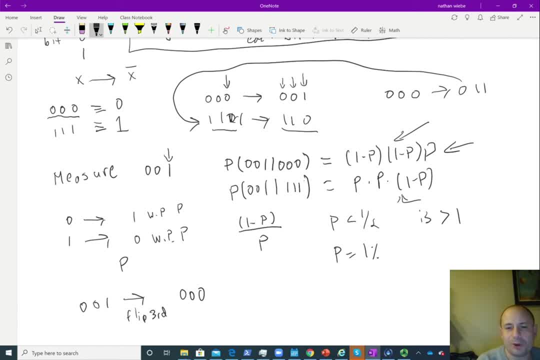 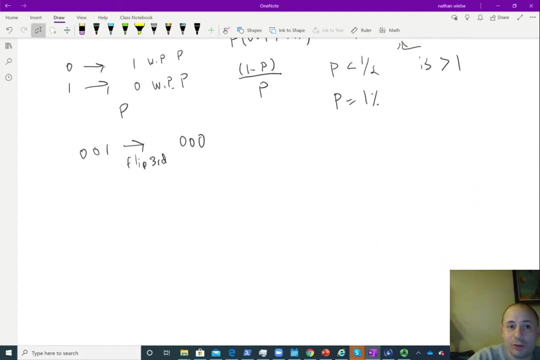 okay, well, 1% is pretty good, But you know, maybe we want more certainty. Is it possible to systematically improve this? And the answer is yeah, it is. So the way that we can do this is we can actually consider more general repetition codes. 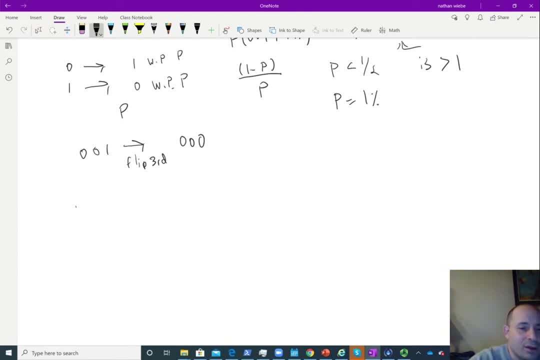 Let's consider having 0 go to 0 to the n and 1 go to 1 to the n. All right, In the event that we end up having this, and let's say that we were to take a look at a bit string. 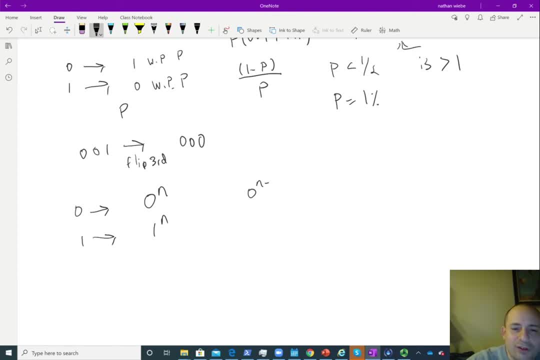 and measure the analog of this. So let's say we measure n minus 1, 0s and the last bit is flipped to 1. Then the probability of generating this bit, string of n minus 1 0s and 1: 1,. 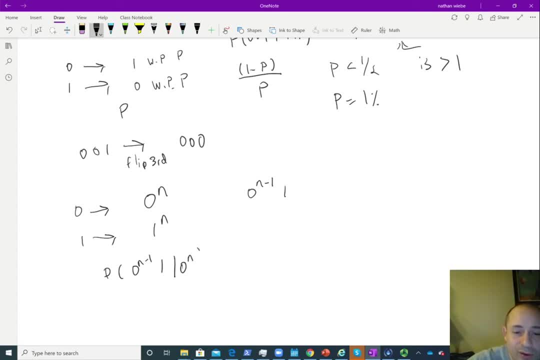 given that the true is 0, true is should have been n? 0s. that is equal to well, just 1 minus p, to the n minus 1 times p, versus the probability of getting the same outcome if the true bit string was n? 1s. 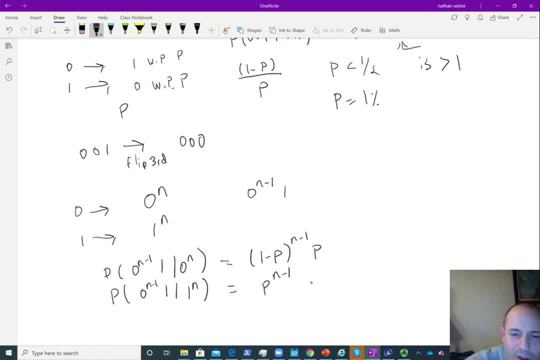 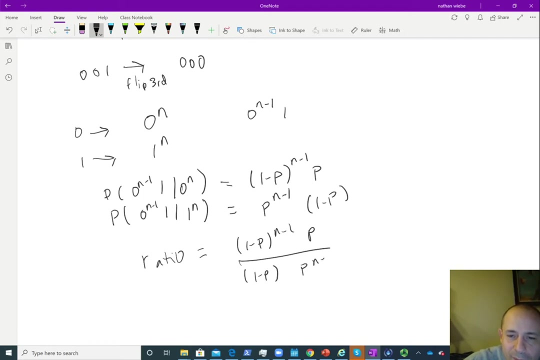 In that case, the probability is p to the n minus 1 times 1 minus p, which ends up giving us a likelihood ratio of 1 minus p to the n minus 1 times p, over 1 minus p times p to the n minus 1. 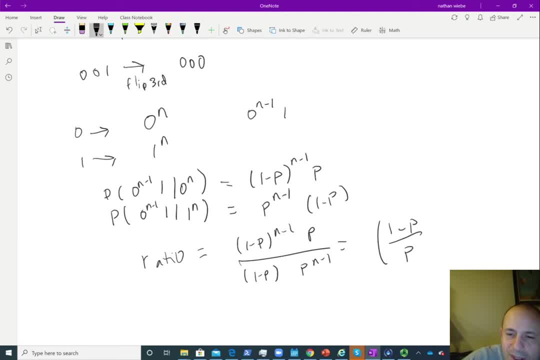 equals 1 minus p over p. now to the n minus 1.. And minus 2,, I'm sorry. So that is how this ends up going And you can see that, provided 1 minus p is less than p, ie if p is less than 1 half. 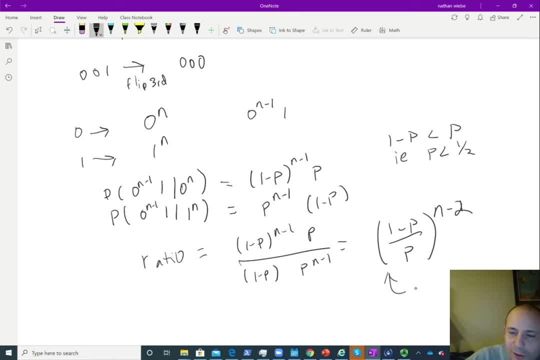 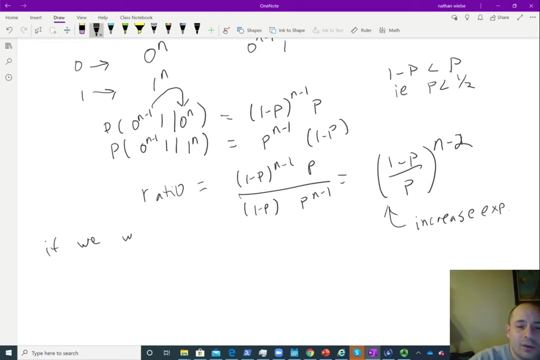 then at that point this likelihood ratio will increase exponentially. So what that ends up meaning is that, with overwhelmingly high probability, saying that this state over here actually corresponds to that one will become exponentially more likely. So what that means is that means that if we want 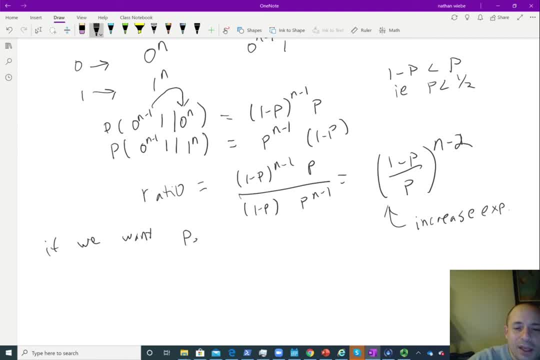 under this error model, the probability of guessing error wrong is. if we want that to be equal to delta, then basically what we end up getting is that, well, delta then is equal to 1 minus p over p, to the n minus 2,. 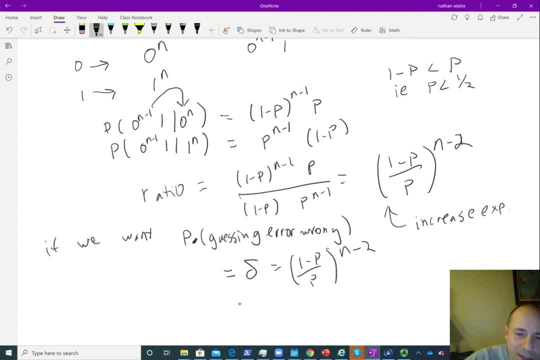 which ends up, meaning that we end up getting or sorry probability. That's a likelihood ratio. I want the probability of guessing incorrectly in this case. So the probability of guessing incorrectly will be p to the n minus 1 times 1 minus p. 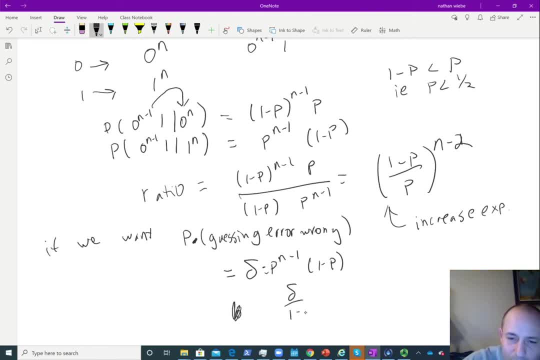 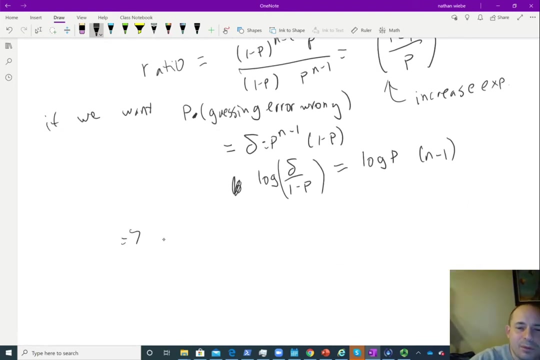 Okay, And therefore we end up getting delta over 1 minus p. log of this is equal to log p times n minus 1.. And so therefore this implies that, taking a value of n in order, log delta over 1 minus p will suffice. 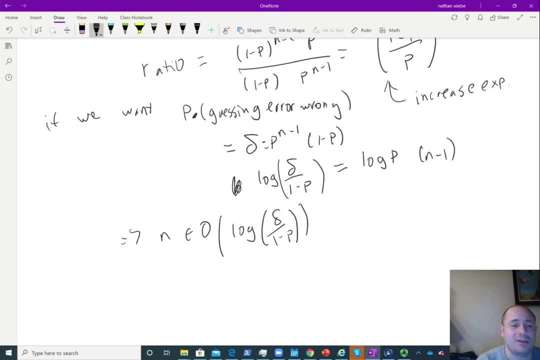 for ensuring that this ends up working. So what that means is that means that we don't require that much redundancy in order to make the probability of us erroneously get a decoding a bit flip error arbitrarily small. So that's fantastic actually, And this is basically. 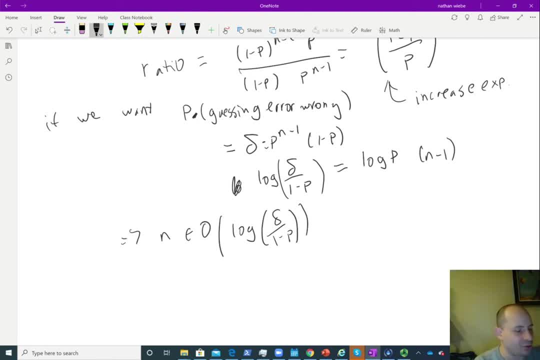 the essence of where the classical stuff ends up getting its power. And, by the way, it should be mentioned that this form of a repetition code is used frequently in ordinary computers for- or sorry, it's used frequently in communication, and also variants of this are used. 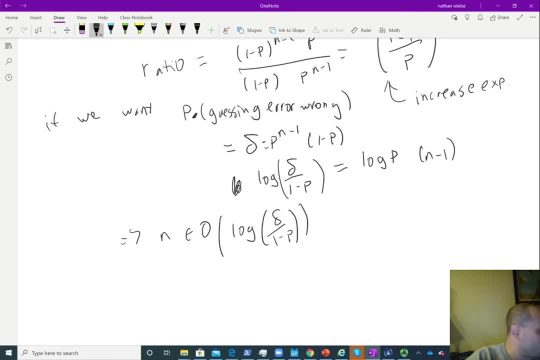 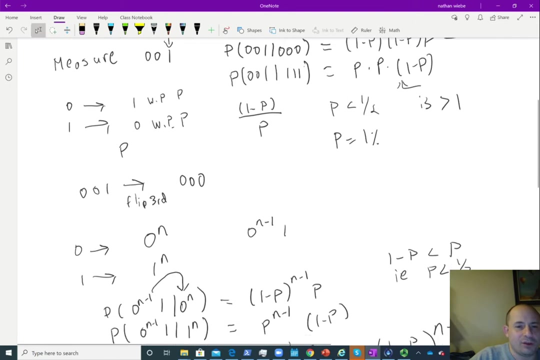 in the parity check protocol. So now that I've discussed this, let's dive a little bit deeper into terminology. Okay, So what we were doing above is we were just exploring what is possible with repetition codes and showing that if we throw more redundancy, 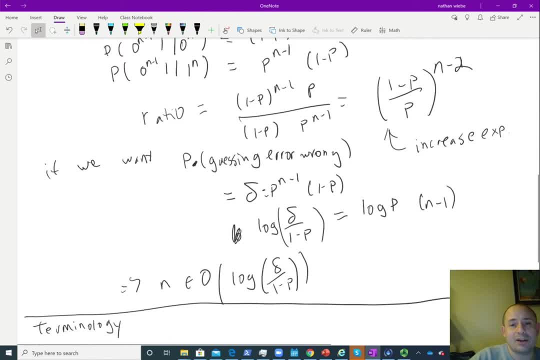 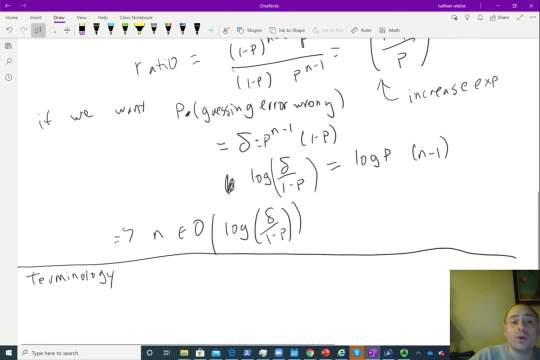 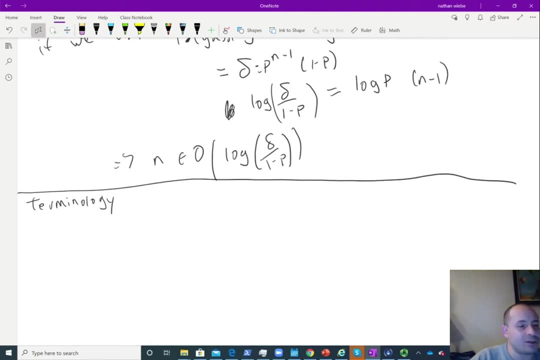 in the repetition code. add an individual problem, then the probability of us incorrectly being able to identify which bit or bits got flipped ends up shrinking exponentially. This actually has something to do with a concept called code distance. So a code has distance d. 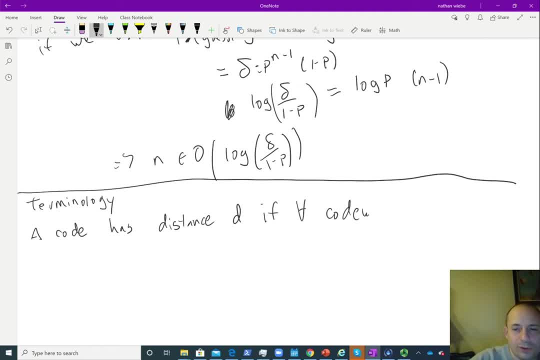 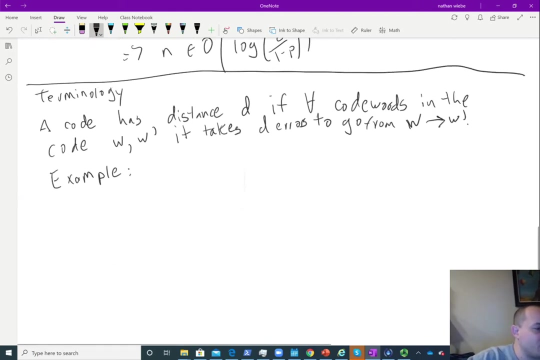 if for all code words in the code w and w prime, it takes d errors to go from one w to w prime. Okay, Here's an example. Let's take a look at the three-bit repetition code that we considered before And again. 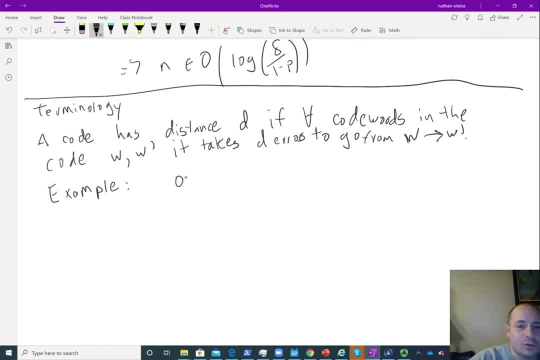 so far, nothing here is quantum. This is just ordinary repetition codes. We have that zero goes to zero, zero zero and one goes to one one one. Okay, This is a distance three code, And the reason why it's distance three is because we need to have an error. 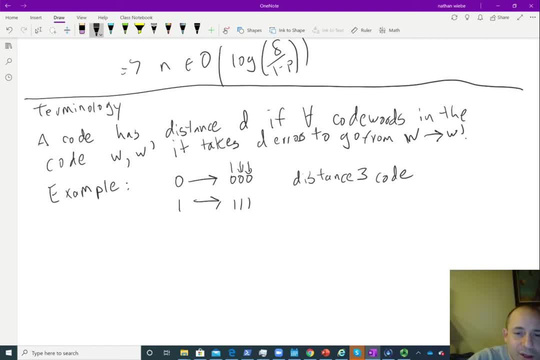 on this site, this site and this site- in order to transform the two code words in here into each other. Okay, So that's, that's why this is a distance three code, And a property of codes is that a distance d code can correct. 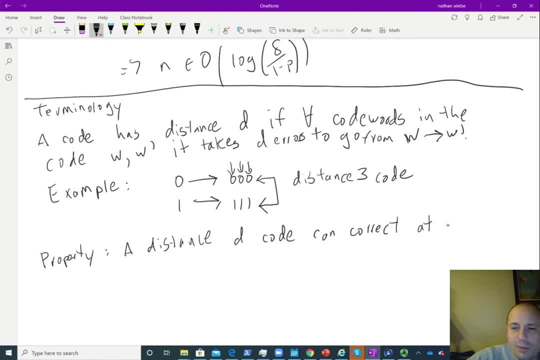 at most, d minus one, over two errors. Okay So, and by errors what I mean is I mean, in this case, flips in the physical bits that end up constituting physical bits, constituting what we call our logical bit over here, which is the. 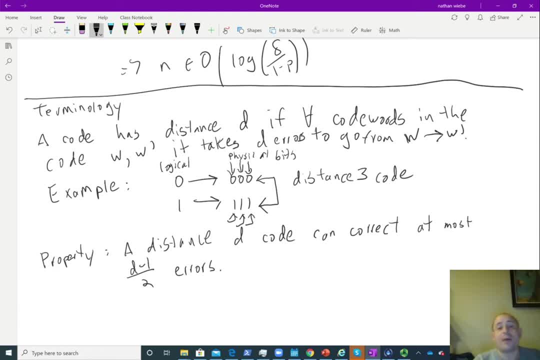 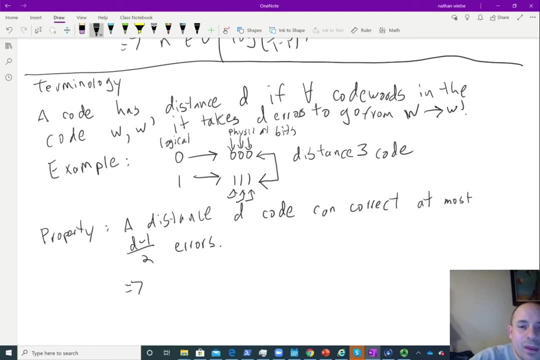 the, the code word, effectively, that we're trying to represent using our physical bits. Now let's take a look at this. We've got three distance. I've got a distance three code here. So this implies that the repetition code here can end up. 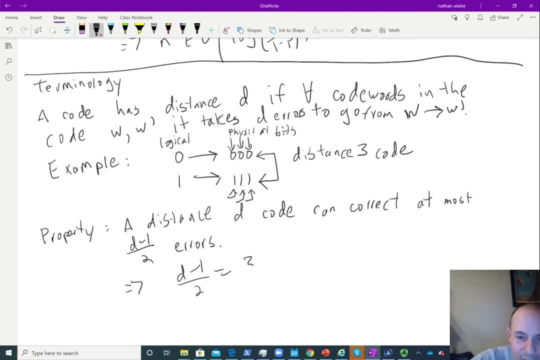 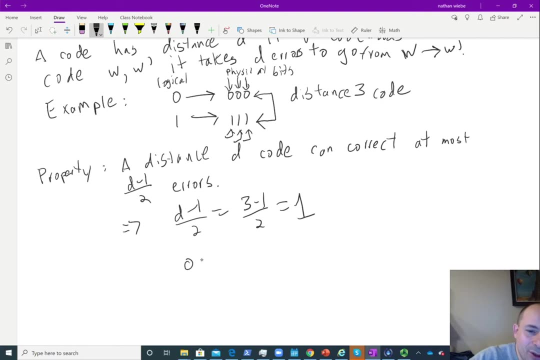 getting. well, d minus one over two is equal to three minus one over two, which is equal to one. So this code can actually correct at most one one error. Why is that, You might wonder? Well, we can see this just by looking at the code. 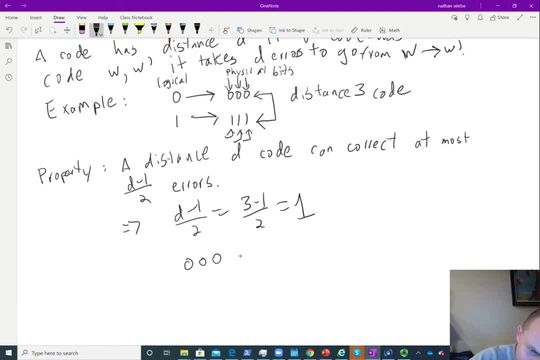 Let's, and also that example that I did previously. So let's say that we were- we're subject to two errors. right, We would map this to zero one one. Now, on the other hand, if we had one one one, 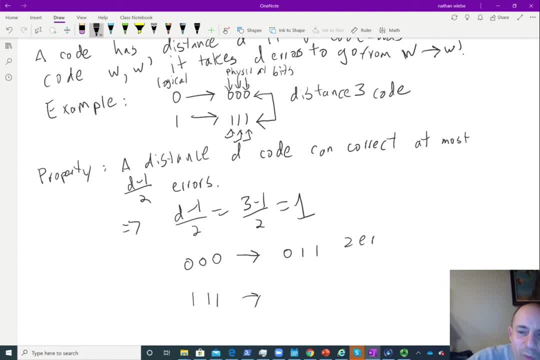 this: the zero, zero, zero requires two errors in order to be able to get to zero one one. However, this requires only one error. So what that means is that means that if we use take the maximum likelihood estimate as the estimate of what error actually happened, 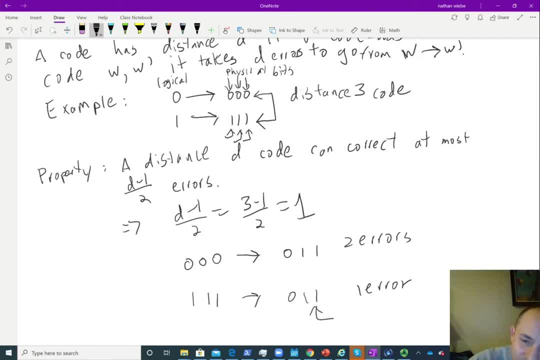 we would say: oh well, it's clearly this one because this is going to be better by a factor of p roughly. However, we, if we knew a priori that there were two errors, we would have made a mistake if we decided. 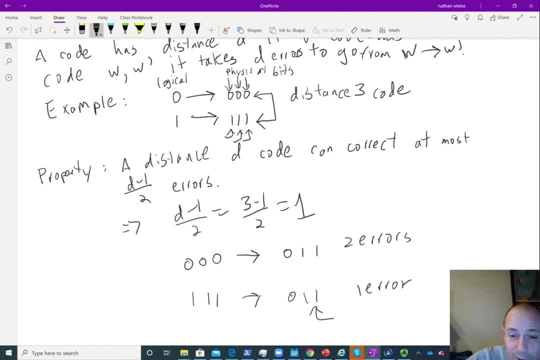 to try to correct this bit flip. by flipping that to one We would have started with our code word zero over here, and by doing that correction we would have mapped it to one. Okay, So that's why we can only correct a distance of d minus one over two errors. 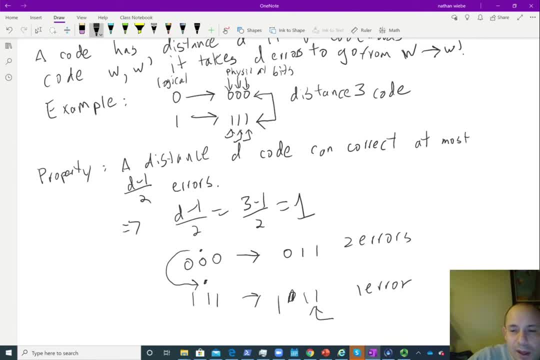 because in the event that we have- basically imagine we just got two code words over here- Once we end up getting a distance in a hamming distance, effectively, in this case, beyond our code word w and w prime- then we start becoming closer to the other code word. 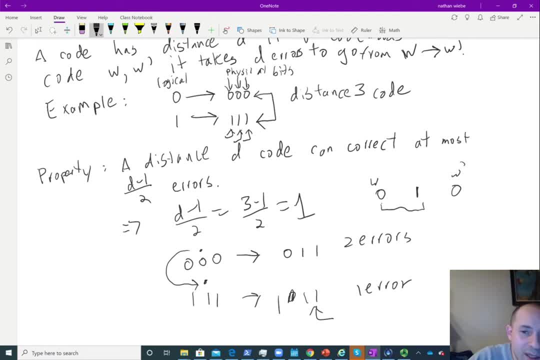 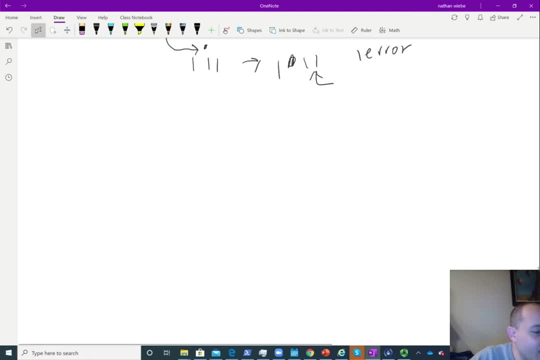 than the previous one, which is why we end up having this property. Okay, So that is. that is. that is what we mean by code distance. Now, often in the literature, you'll end up seeing the following notation, And I just wanted to mention it: 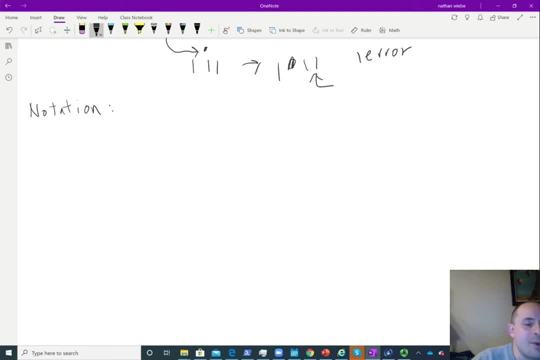 because sometimes it it can show up and trip people up. We could say that a code is called a N K D code if it uses N bits to encode K bits with distance d. So, for example, the code, the repetition code that we considered above, 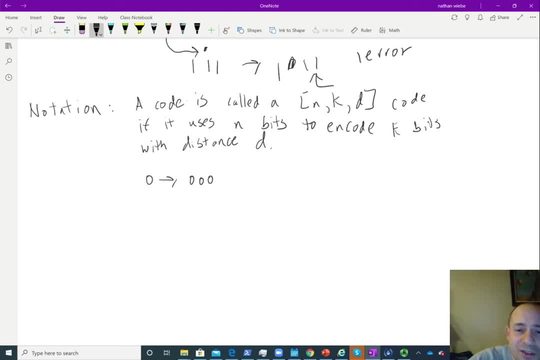 you know, which is just zero going to zero, zero, zero. This has an N of three over here, It has a value of K of one because it encodes one bit And, as mentioned before, it has distance three over here. 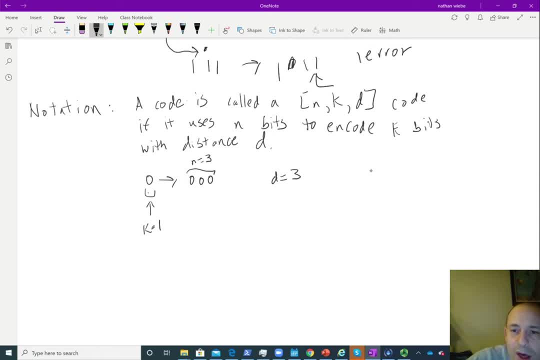 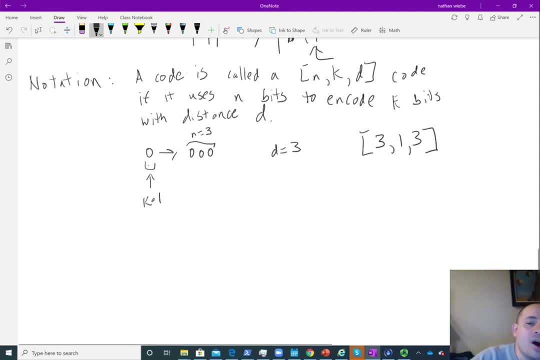 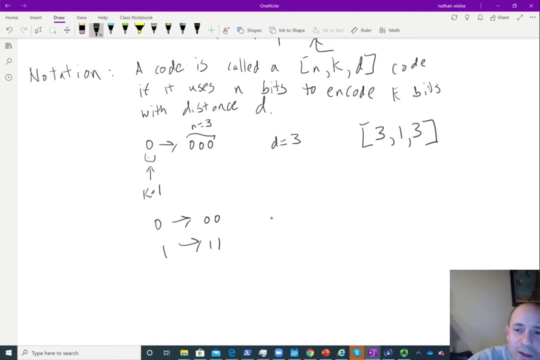 So this would be an example of a three, one, three code. Okay, Now, on the other hand, if we ended up having the simpler code: zero goes to zero, zero and one goes to one. one, the distance. 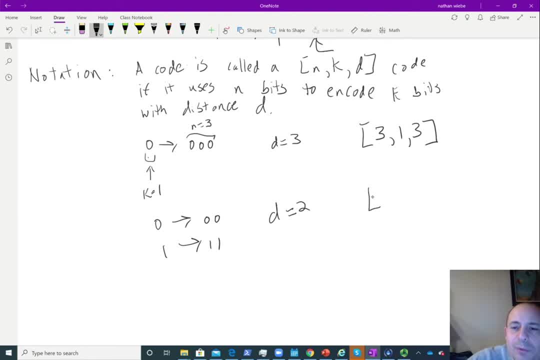 would be equal to two in this case, And that would correspond to a two one two code. Also, I should mention, in this case we cannot correct errors. However, we can detect the presence of them with this code. 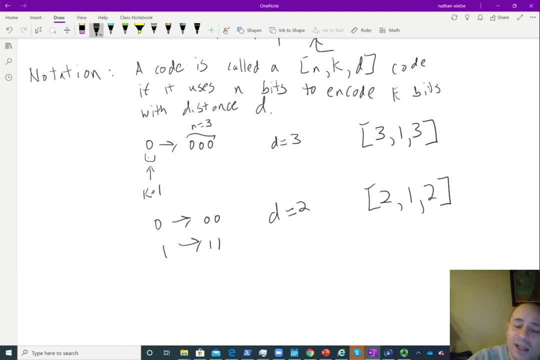 So even codes that can't correct errors, like this one, still can be useful, because sometimes they'll let you know that an error in fact happened. So that's, that's basically it And the in general, as I mentioned before, 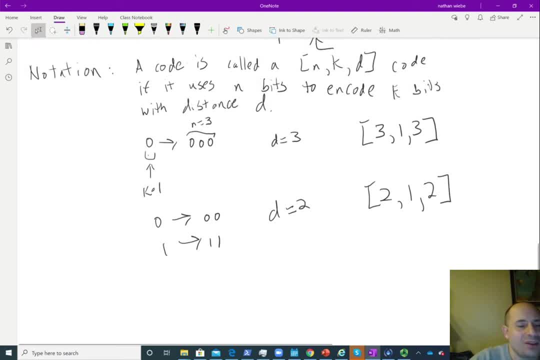 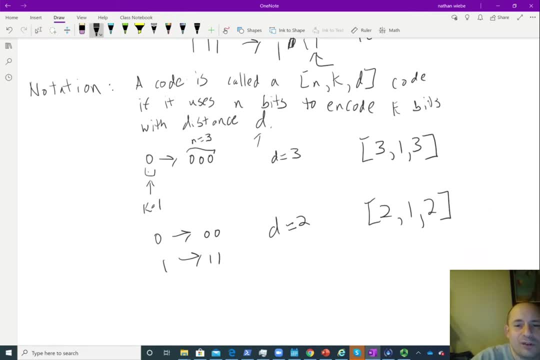 the probability of having an error that you can't detect or correct using these schemes shrinks exponentially with the code distance over here. So that's basically how class the classical case ends up going. Now, quantumly, what we're going to want to do. 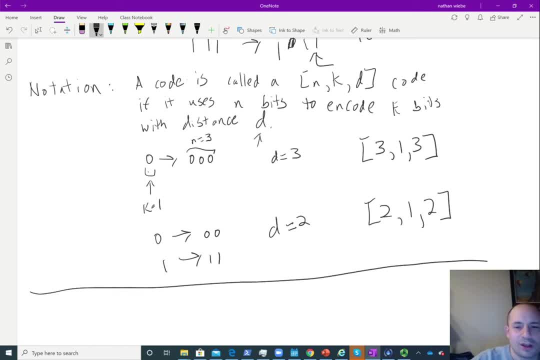 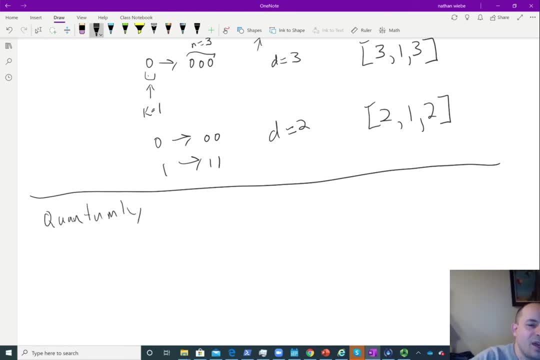 is. we're going to want to deal with a couple of challenges. Quantumly, the biggest challenge that we're going to want to deal deal with- and people actually thought that this would be a deal breaker to begin with- is the problem of measurement. 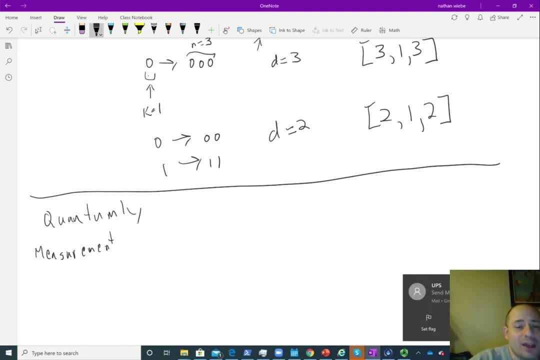 So if we ended up having a state, let's say zero, and I'll be very clear: often what we'll do in quantum error correction language is we'll put an L down here to mean that this is the logical state corresponding to a physical. 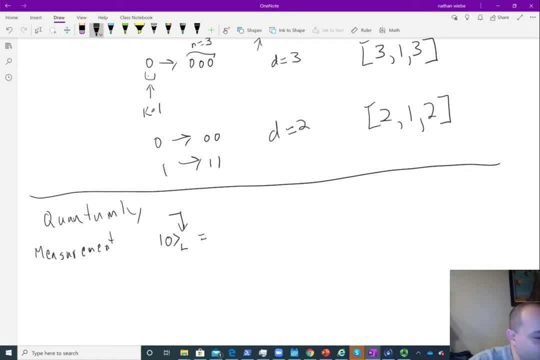 state: Okay, This for the, if we were to try to use the repetition code, would be just say zero, zero, zero, And we'd have one logical equals one, one one. So this is the exact same thing. 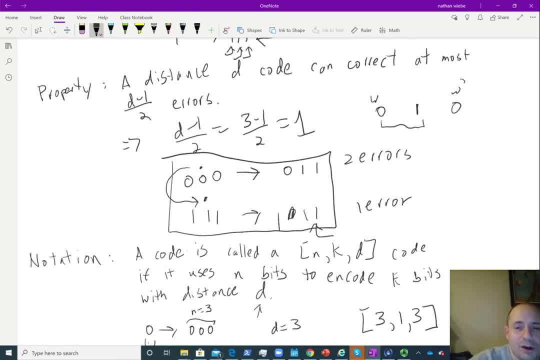 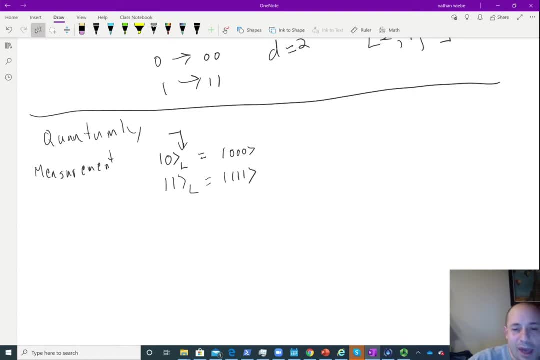 that I ended up doing with this rule here, except I'm applying the same thing in the quantum world. All right, So let's say that what we have is we have a bit flip, Okay, And the way that we would have this is: 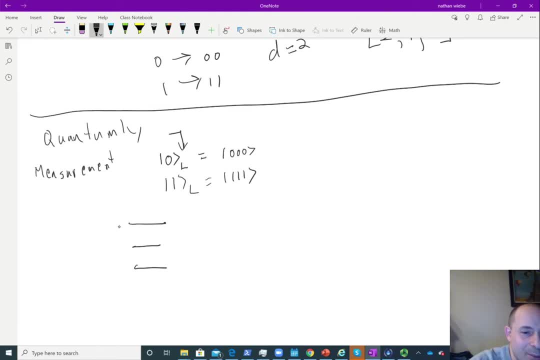 we would could envision this as a quantum circuit. Ideally, we'd like to be able to do the, let's say, zero, but we have an error over here, which is an X gate. This is an error We don't want. 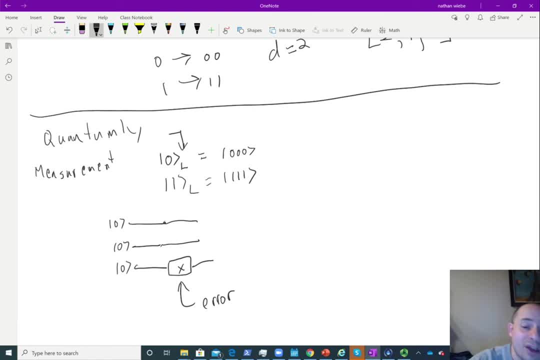 to have this X gate, but because of a hardware imperfection, that bit got flipped partway through. Okay, So what we would like to be able to do is we'd like to be able to detect it, So we could just measure. 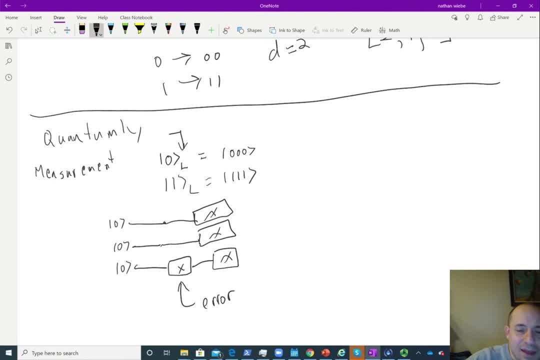 All right, All of these at the end, and then we would end up seeing that flying out of this comes zero, zero one. Well, let's fix that, then, just by simply re-preparing the state. well, zero, zero. 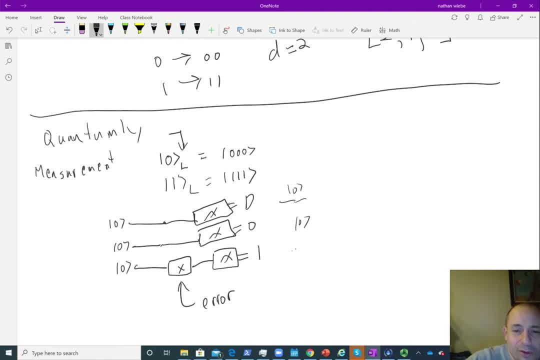 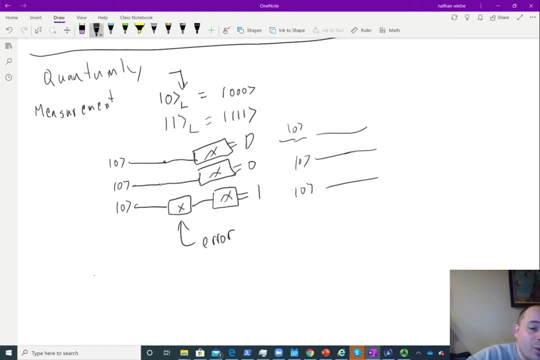 zero over here and done. Life is good, right, But what if our state was of the form a zero logical plus zero logical plus b one logical, which is equal to a zero, zero, zero plus b one one one? Well, 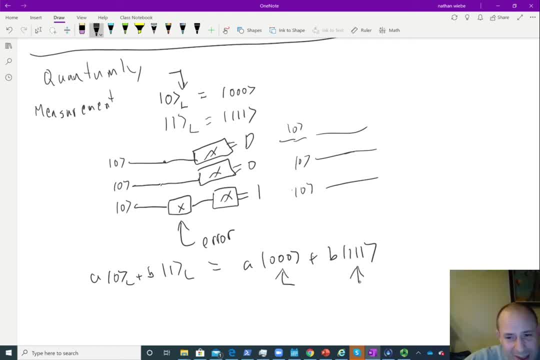 in the event that we measured all of them, we would project to either this case or that case, thereby damaging our system. So, at first glance, because measurement of all of these different bit strings over here seems to give us information about which possibility we're going through, 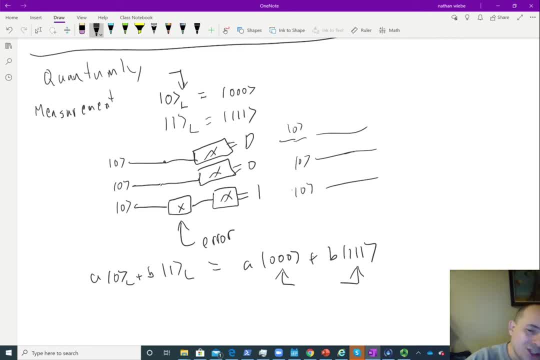 it seems at first glance that error correction actually is entirely antithetical to the idea of quantum computing, But actually that isn't true at all. In fact, there we can measure all of this information without revealing any of the salient information about the. 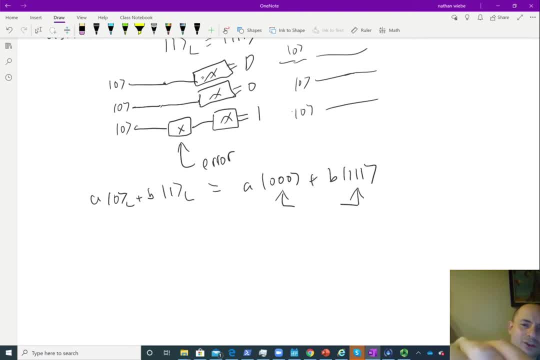 the bits. For example, let's now just go ahead and look at what ends up happening in this case, where we end up putting now our state psi in through this circuit. Well, what we would end up getting out is we would get a zero. 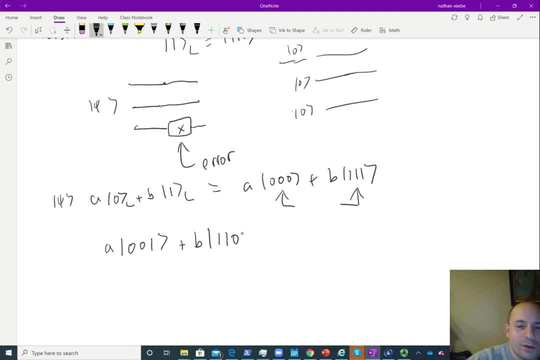 zero one plus b one, one zero, Okay, Fantastic. So now, obviously, if we measured every single bit we would be able to, we would learn whether we've we're on this branch or that one. Instead, let's take a look at a different property. 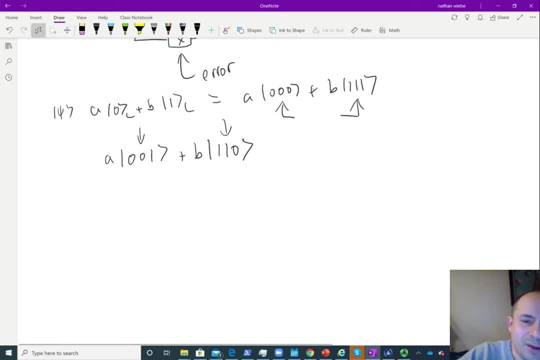 Let's take a look at the parity between the individual bits. So if we instead measured the parity between these two, the parity of these two bits would be zero, exclusive or zero, and one exclusive or one that's equal to zero. That gives us no information. 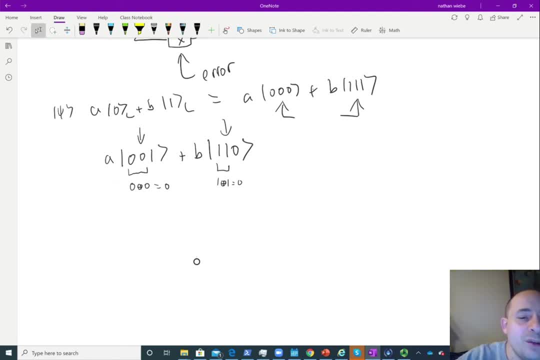 about whether we're on this side or that side. So we could. we could measure the parity just fine, without distinguishing those two states. Okay, Great, Now let's envision that we do the exact same thing and we measure those parities. Well, in this case, 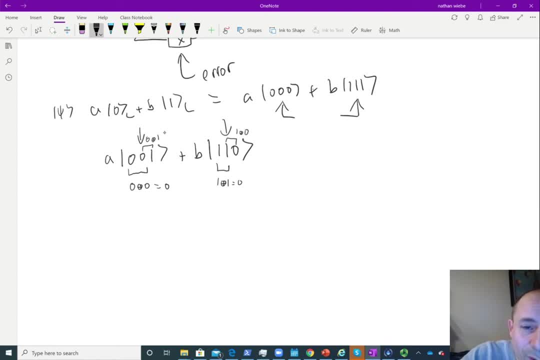 we would get zero exclusive or one, and one exclusive or zero. so by measuring the parity, we would have learned, in this particular case, that these two bits have the same value, but those two are flipped, And so what we can do is: from this information we can infer: 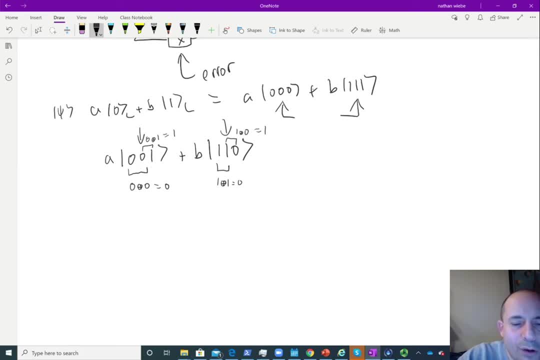 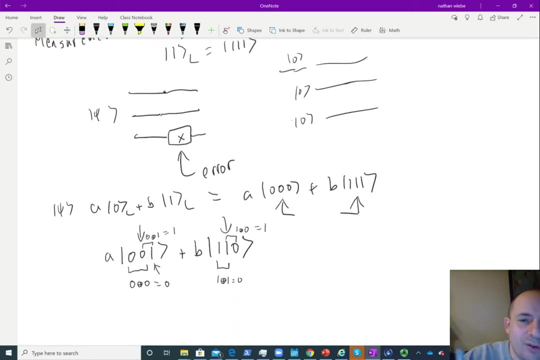 oh well, if these two are consistent and that one is flipped, then the most likely model is that this qubit ended up having an x error associated with it. So what we would do in that case is we would begin with some block that would measure parity. 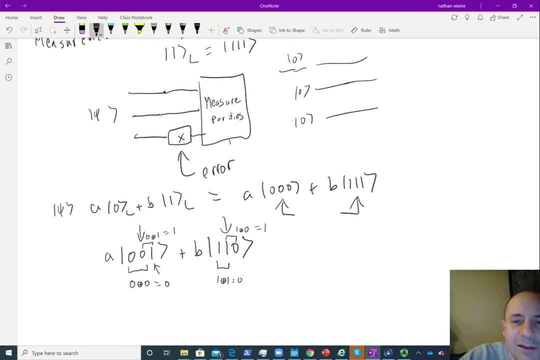 or the parities of all of these individual bit strings, and based on these particular outcomes, what we will do is we will apply, in this case, a controlled, we will apply an x gate to flip that third qubit where the error ends up happening. Okay, 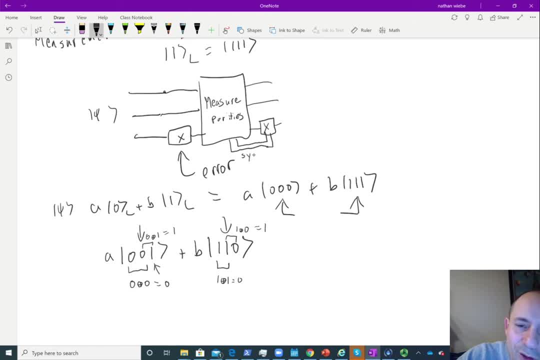 This data over here is called an error syndrome. Okay, Just like we talk about illnesses being syndromes, we use the same terminology for errors. This information, through the parities, ends up coming back and allows us to work backwards and figure out what the most likely. 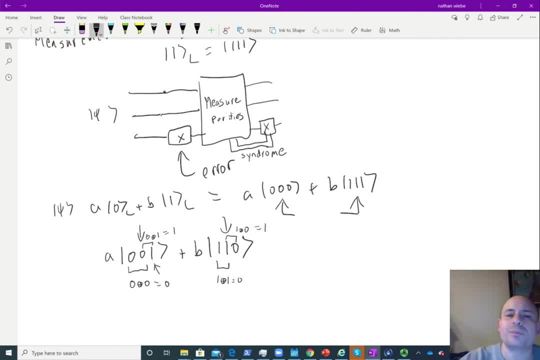 error is, and then we can correct it. It's important to note physically, though, if we were carrying this out. this error correction step requires inference from the syndromes to figure out what the correct in general correction block that we should put in afterwards in order to deal with it. 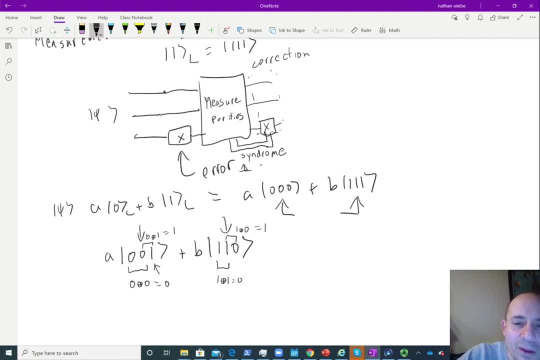 This part over here requires substantial- not as substantial as it once did, but it still requires substantial compute to make this happen. So in practice, what ends up happening with quantum error correction is that you kind of have this hybrid system where a you, you're getting an ordinary. 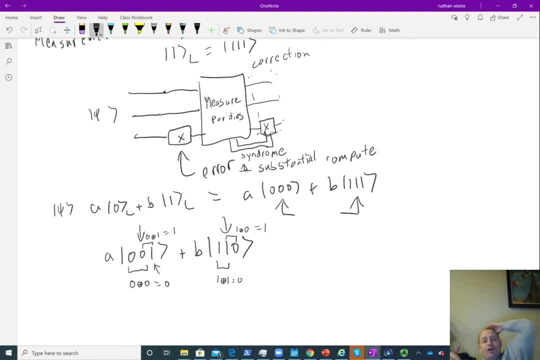 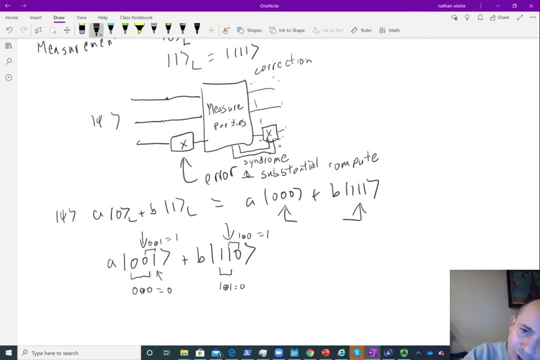 classical computer to process and interpret the measurement outcomes from the quantum computer and then figure out what the most likely errors are and intervene and correct. Okay, So that's the idea and, incidentally, in practice actually often these error, these x gates over here aren't even 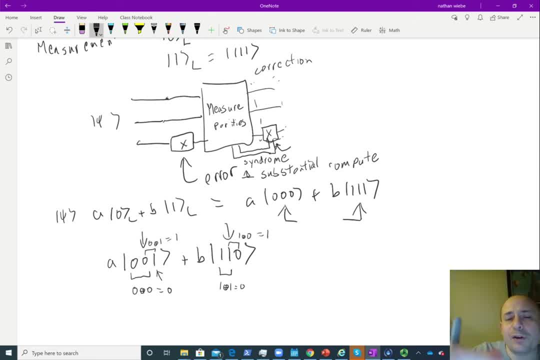 applied In practice. we just redefine our frame of reference and recompile the rest of the calculation around the fact that we know that this bit has been flipped, And that way we can save any errors that would come in by trying to flip the bit again. 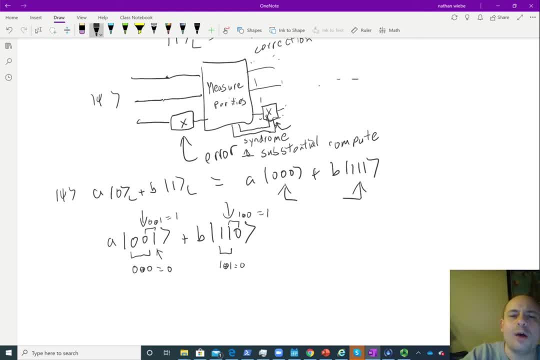 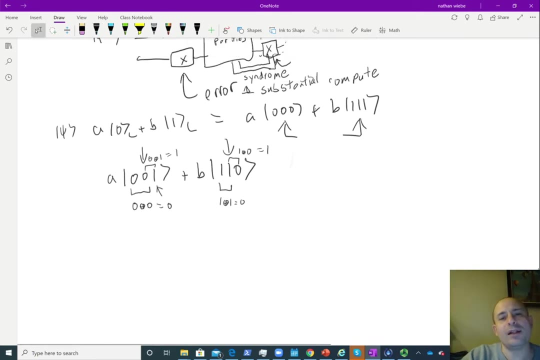 So that's just a. it's kind of a cute trick that people do in practice, but at a high level. we can always envision the error correction operation as physically correcting each of those individual errors. Okay, Cool. So now that you've got an idea, 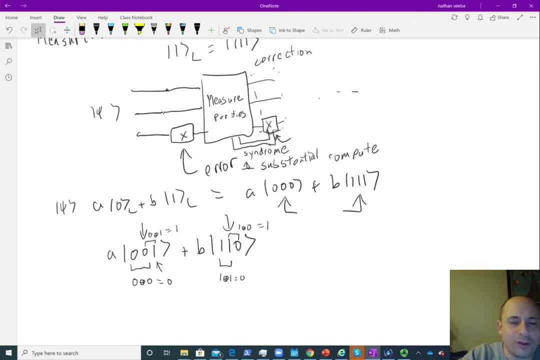 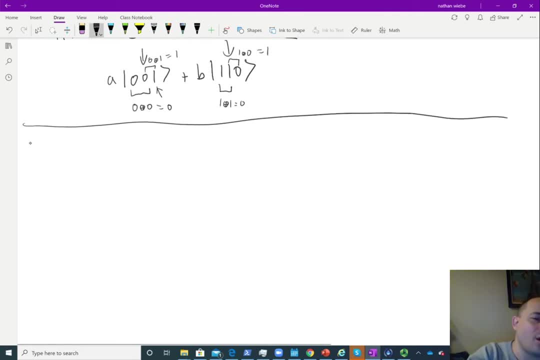 about how all of this works. I'm going to zoom in a little bit more on several of these these steps. So basically in every error correction protocol there are kind of three stages. The first stage is the encoding stage. Second is the syndrome detection slash. 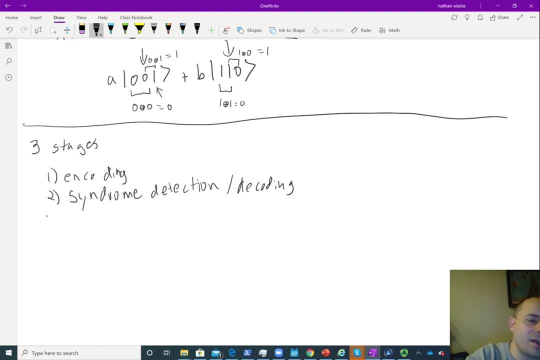 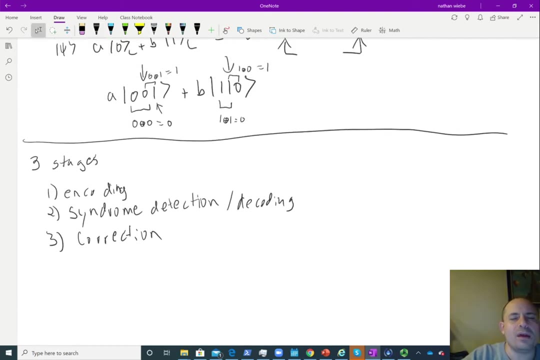 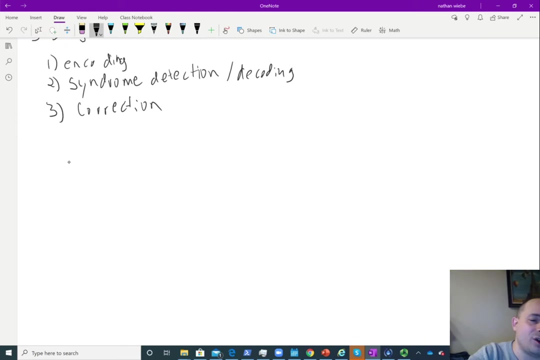 decoding phase And then the third one is the correction. Okay, So let's just deal with the encoding phase and, specifically looking at this, this repetition code that we've been talking about. So the encoding procedure for the repetition code is actually as follows: 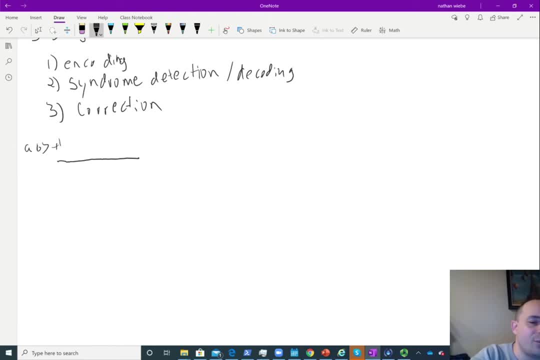 So let's say we start with a state- a zero plus b one over here, and we want to encode that in our system. We're going to begin with two quantum bits over here set to zero- Now the most, the easiest way to do this, and 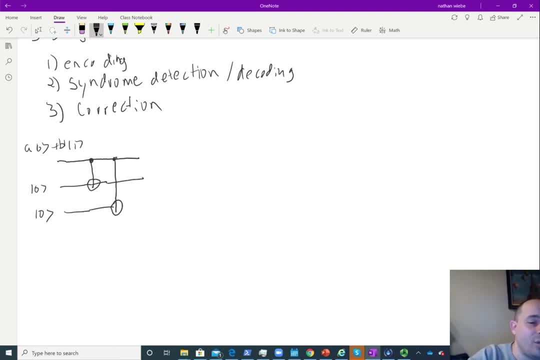 perhaps most natural is this over here? Okay, So once we end up doing this, then it's very easy to see what the state that we would end up getting out the other side would be: a zero, zero plus, Okay, cool. So now we've encoded this, Since both of these are our code words, you know. 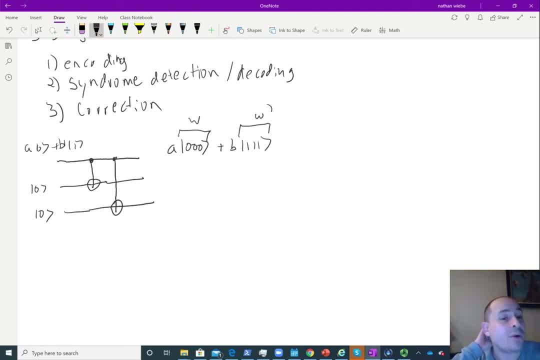 they're like W and W prime. using the above discussion, we've now encoded this inside our quantum error correcting code. Okay, cool. Now there's some other options to this that I should mention need to be thought of in order to make this happen. So another option: 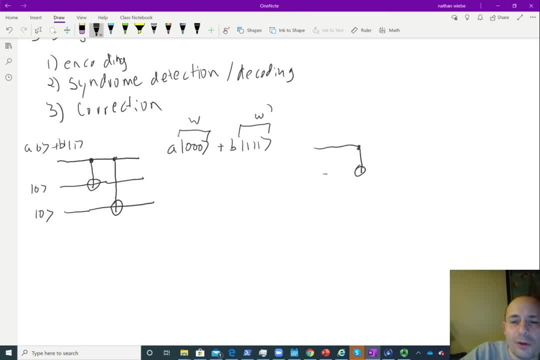 that we could have done is we could have considered following circuit for encoding: Okay, this over here. Now, both of them will end up mapping A zero plus B, one zero zero to the exact same thing over here, But within the error model that we've posited. 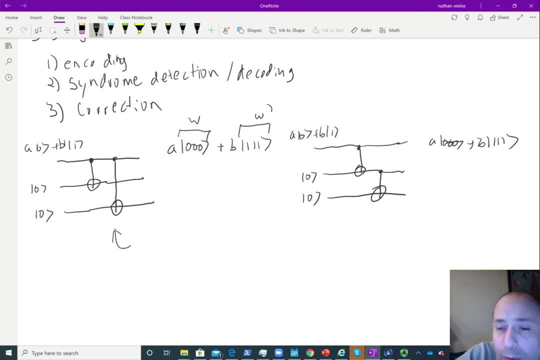 this one actually is way, way better to do than that one, which seems kind of strange because physically they look very similar And, on top of that, because this one's only using nearest neighbor interactions, it looks like this might be even easier to engineer. 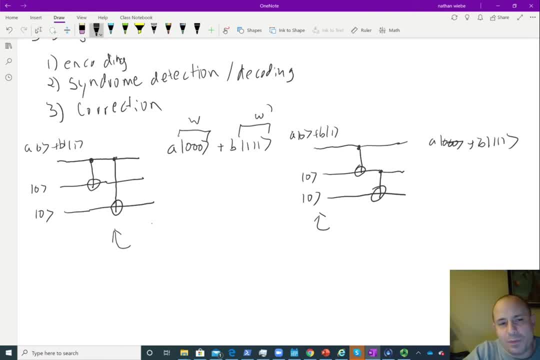 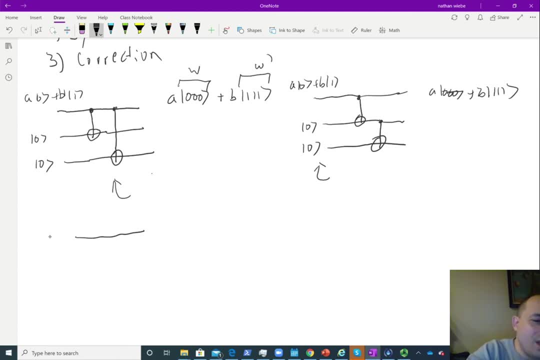 But despite that, this is actually the better option. The reason why can be seen as follows: Okay, let's look at the simplest case. Let's look at the case where we have. Okay, let's look at the simplest case. Let's look at the case where we have. 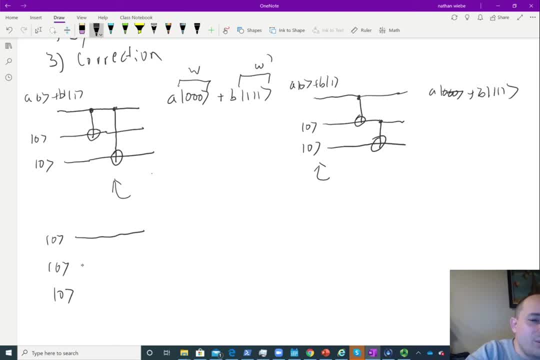 an error on the third bit. Okay, we can always envision that error occurring in the following way: Let's say that there's an X gate that ends up flipping it. Okay, now if we do the same thing over here, we can end up seeing that this will have the exact same effect as 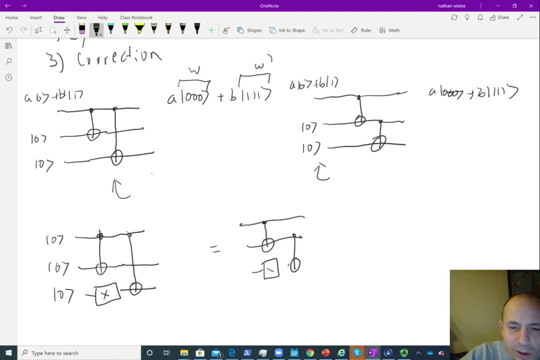 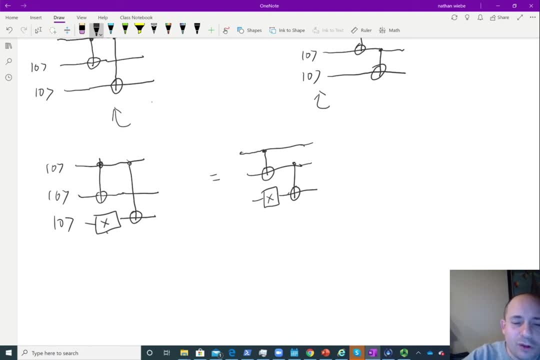 this over here. The reason why these two are equal is because of the fact that not commutes with control control not, at least on the target. So therefore this is equal to and, by the way, commutes, two matrices. again, commuting means AB. 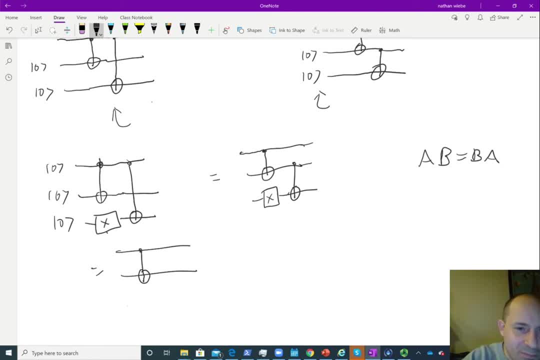 equals BA, so we can switch. the order is all I mean by commuting. So this is equal to the same. actually, E to the power zero. Okay, Thank you. Anything else, That was neat. Yeah to that. similarly, this is equal to this over here. in both cases we have one error coming in. 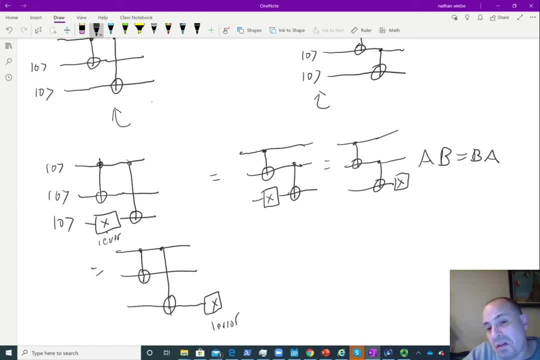 and we've got one error coming out. all right, cool, so it looks like they're kind of the same. but now let's assume this error happens in the second qubit, not the third. so in that case what we would end up having is we would have x control not and x going down here. 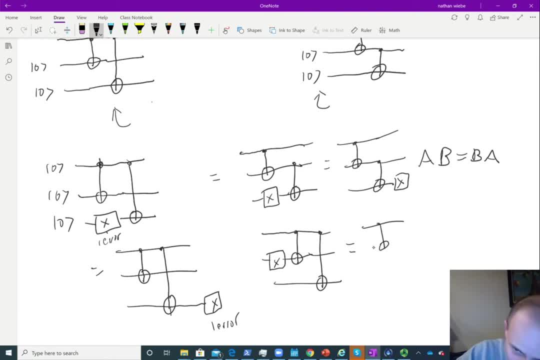 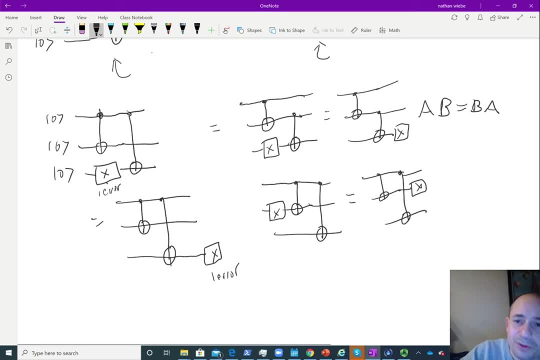 and this one, using exact same logic, will end up giving us one error popping out the other side. now, if we do the same thing with the other case, we would end up having x coming in here, going down there. now. x does not commute with the controls of a, c, not gate. 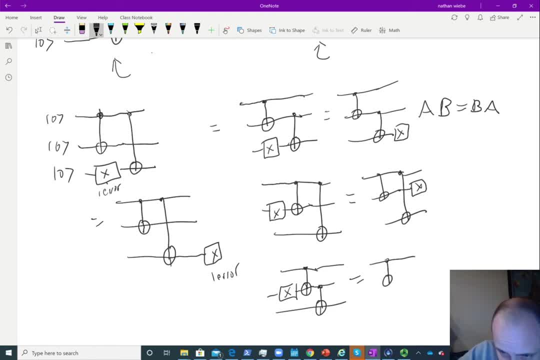 using our circuit identities, we can end up showing it. this is equal to that. so in this case, two errors come out, and so this is a bad, bad thing to have if we want to have a- uh, a encoding that's robust to bit flip errors, because of the fact that it has this: 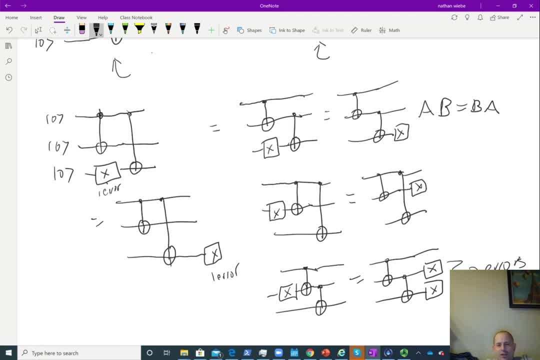 possibility for one error on the input to end up propagating to two errors on the output. so that is um. that is why this circuit over here is generally considered to be the better option. uh, in general, what we want is we want to have circuits cookies pick up that mimi signal over here, over here. and I want to leave a distance from this coil because the pi's loop holders a value over its input value and then, along this line, хочется up on this mimi. 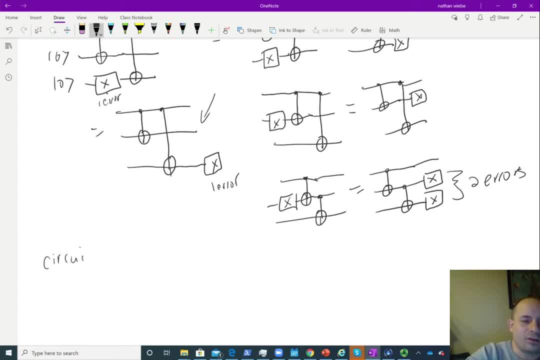 have circuits. circuits that don't necessarily propagate errors are called fault tolerant, And a lot of the work that in comes in to the quantum error correction field is really boiling down to finding good circuits that can tolerate errors of this like this. Okay, so what we want to? 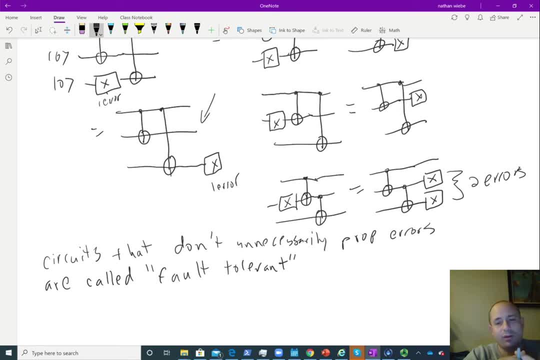 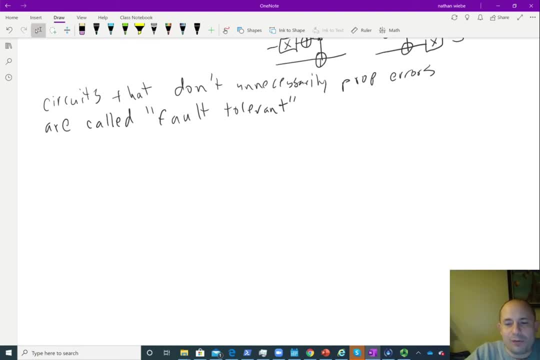 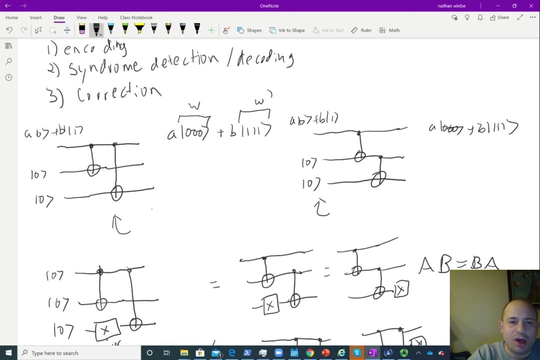 do is we want to build up fault tolerance in our encoding and our decoding schemes, So that is how encoding ends up working. For the repetition code, we basically just end up using a transformation of this form over here in order to be able to take an input state in an unencoded 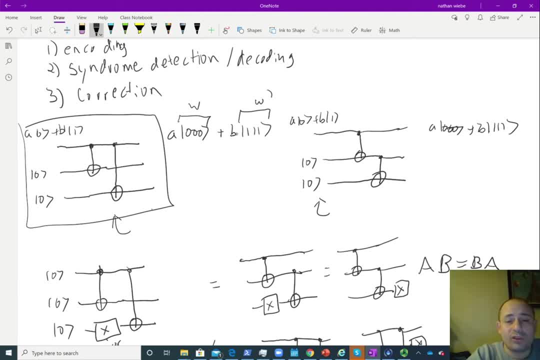 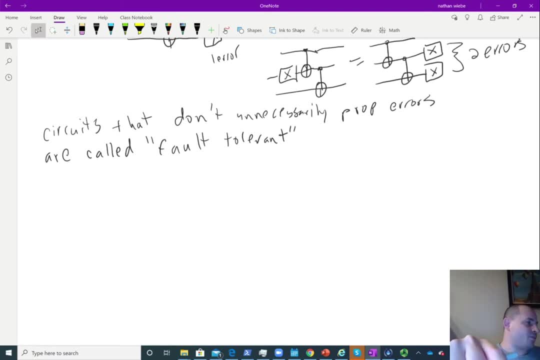 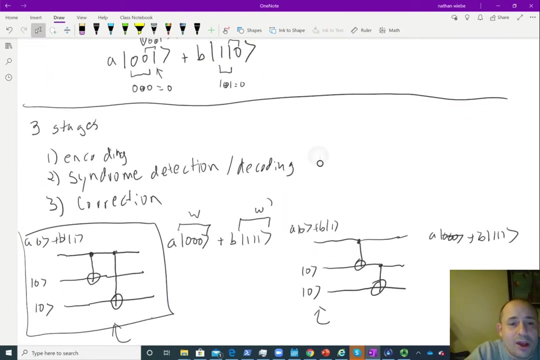 form and then transfer it over to its encoded version. Great, now let's take a look at the. let's take a look at the next aspect of this, which is: we would like to be able to measure the syndromes, ie decode these values. 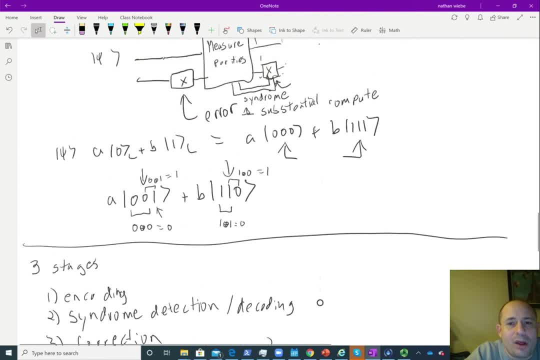 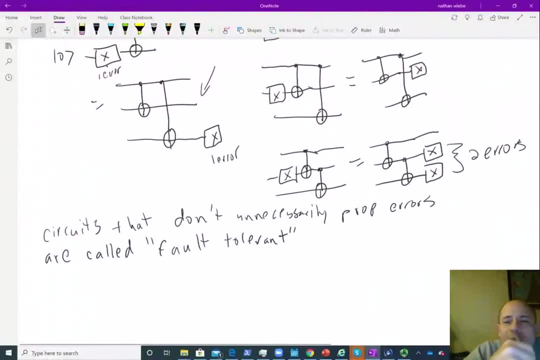 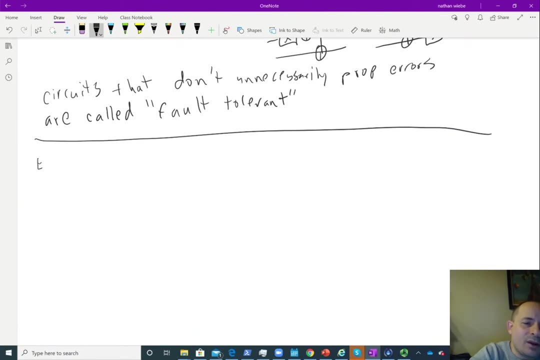 So there's a number of different ways that we can end up doing this. Now, the way that I prefer to think about this is that let's envision the error detection, slash, decoding step. Okay, so say, we've got a situation where we have, you know, our 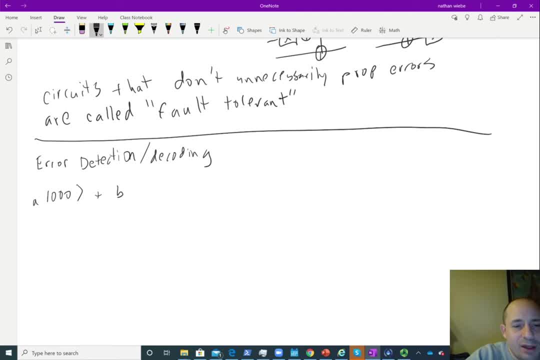 repetition code, which is, you know, our qubit, encoded in the three one three code is going to be this over here. Now what we we can do is we can take a look at the decoder and find where we've got two errors, and then, Right, let's say we take a look at the different types of physical errors that we can end up having. 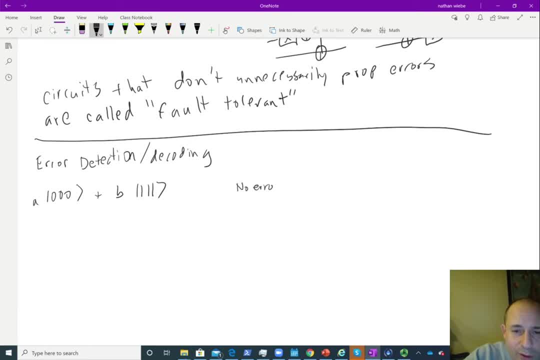 We could have no error. We could have one error. however, we can never have two errors because in the event that we have two errors, as we said before, Well, our decoder will end up saying it's more or less the same error, but it actually wondering if it's. 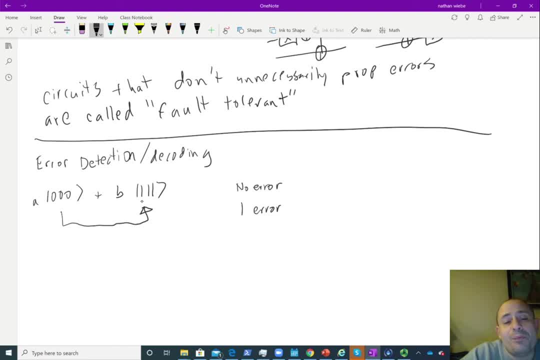 it's more likely that the code word that we're seeing came from the other side. So that means that we only are going to have to worry about these two cases over here, because the two error case can't be handled by this distance. three code: 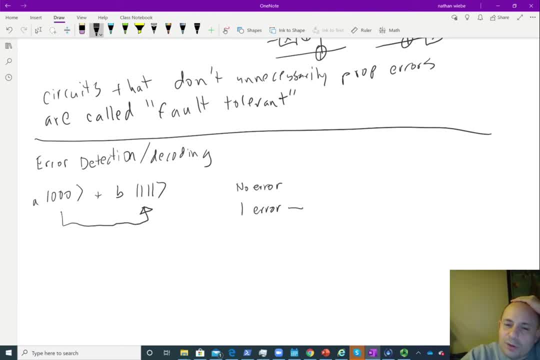 So we've got no error and one error. There's actually three possible errors that we could end up seeing for this. We could end up seeing an error on the rightmost qubit, which would be given by an IIX operation. We could see an error happening on the second one. 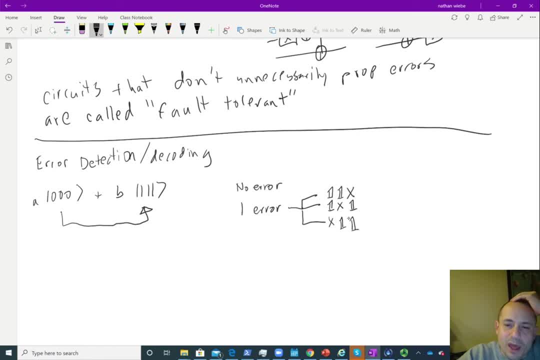 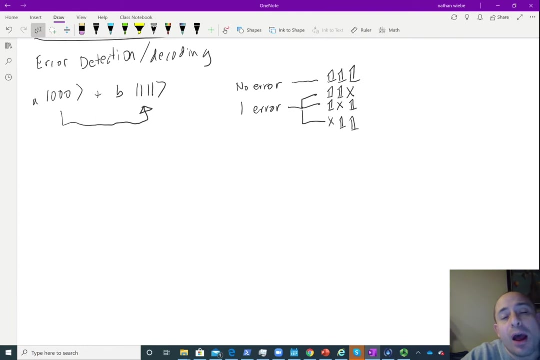 or we could see an error happening on the first one And, of course, if there's no error, that corresponds to the identity transformation being applied to all three qubits. So that is what we would like to do. So if that's the case, then what we can do is we can consider: 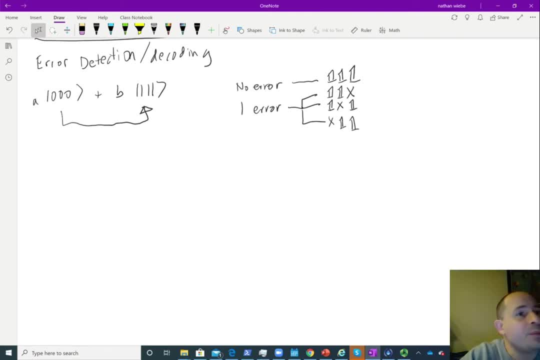 a projector onto each of these different cases in order to be able to see whether or not we have, say no, errors. So a projector which we can use- I'm going to call it p hat zero- that is going to be able to project us onto the zero error space, I can write as the following matrix: 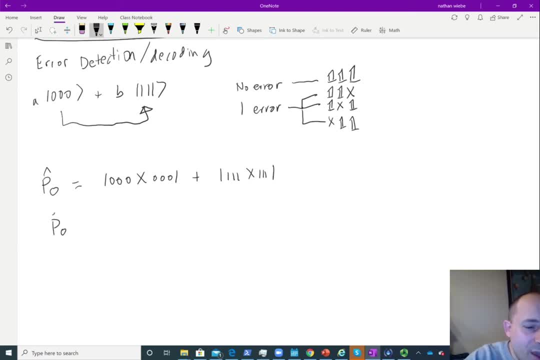 And now this has the property that if we take the no error projector and act it on the quantum state that we assume or the ideal error free quantum state that we have in here, this will end up giving us actually just A zero, zero, zero, because this is the only term that 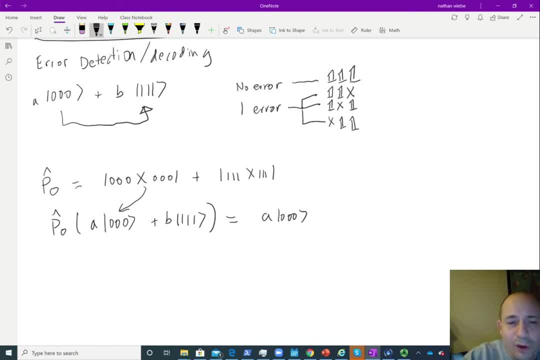 ends up hitting that And this and that have inner product 1.. So that ends up leading us to that plus B 111.. So we can see that this projection operator- no error- acting on this state over here actually really corresponds to honest to god, the real estate that we want. okay, great, so that would. 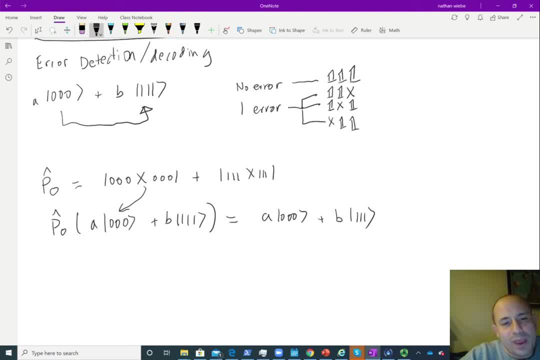 be the no air projector, and so if we uh want to to do this, basically, what we would like to do is we'd like to find some way of implementing this projector or other projectors like this. similarly, we can define the error: um, i'll call it. i i x, meaning the projector. onto this case over here. 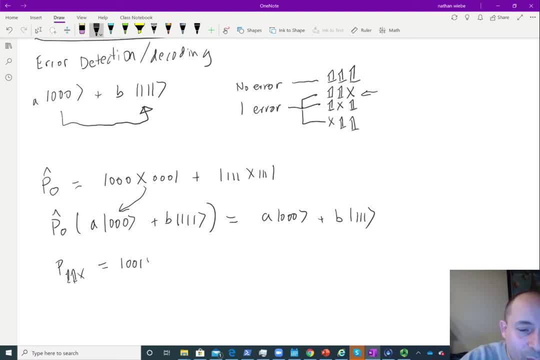 that would be the projector: zero zero one, zero zero one plus one one zero one, one, zero. okay, and so that is how we can um build these things up and by applying or measuring these projectors, we can identify which of these individual error spaces we're in. furthermore, actually measurement of them is. 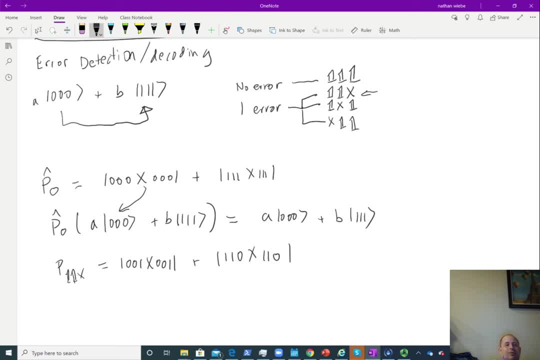 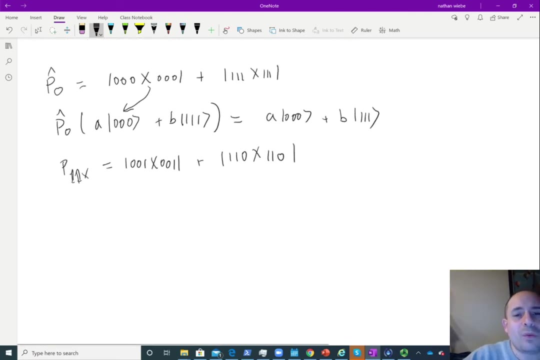 actually going to project us onto one of those spaces and that will give you a bit of a hint about how we're going to be able to handle generic errors when we go forward and talk about the shore code, which is a generalization of this idea. but in any case, this is what we would like to do now. problem is is that i haven't really discussed 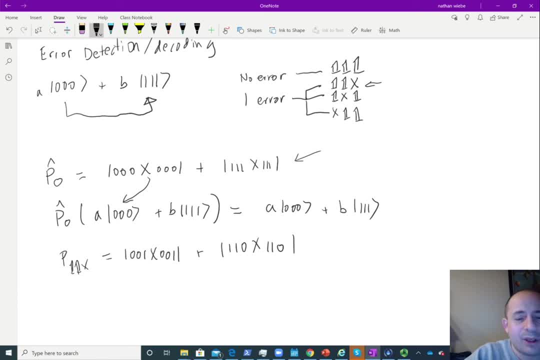 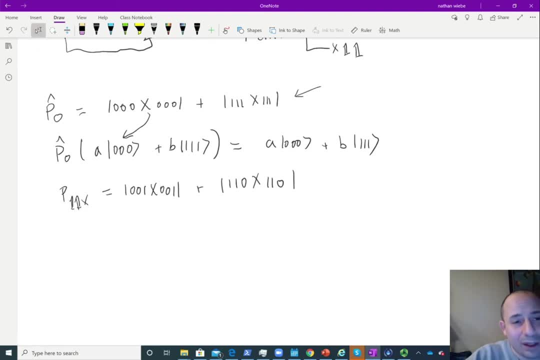 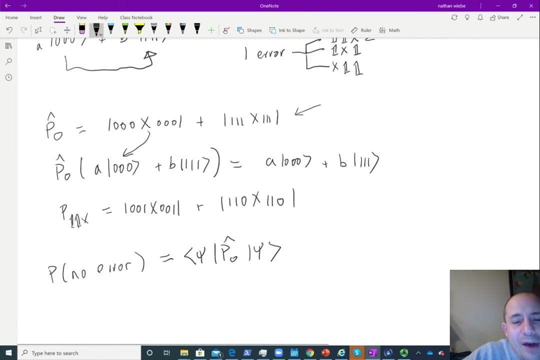 how we could measure the x, uh, how we could measure a projector directly. right, we've already discussed how we can figure out the probability of some configuration, the probability of no error. for example, for an arbitrary state, psi is equal to zero. psi, p naught hat psi. so that is, we have worked with these sorts of objects before and we 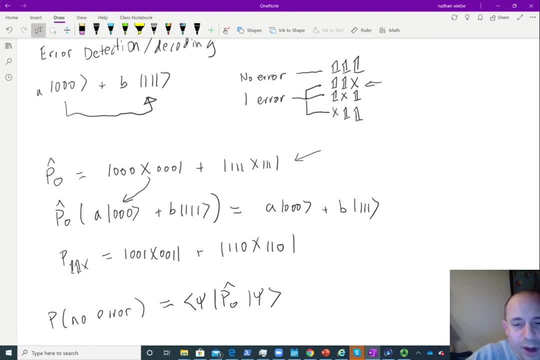 can figure out what the problem for a particular system, what the probability of measuring no error um in our output qubits is. it's just this guy right here that probability, or, sorry, that projector still haven't described how to operationalize. so let's take a look at building this particular. 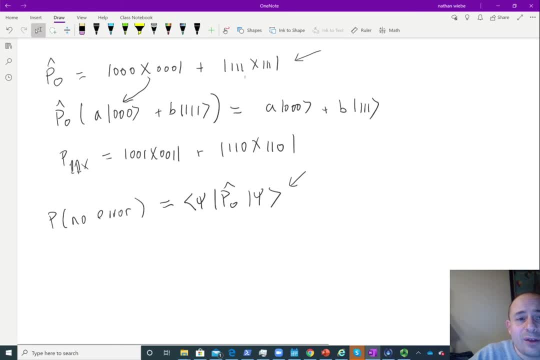 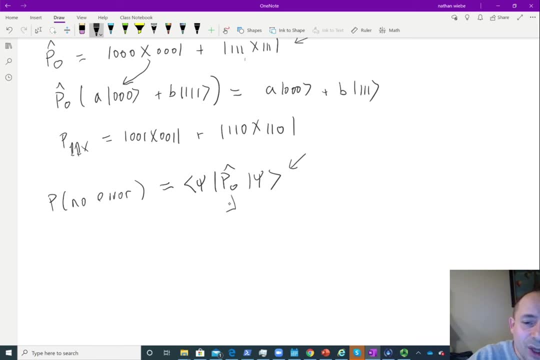 projector. the easiest way to do this is what we would like to do- is something. let's say what we could. we could do is we could write the projector: p naught hat is equal to a? u 1 plus b? u 2, so on and so forth. and this over here i i'm going to call a linear combination of unitaries. 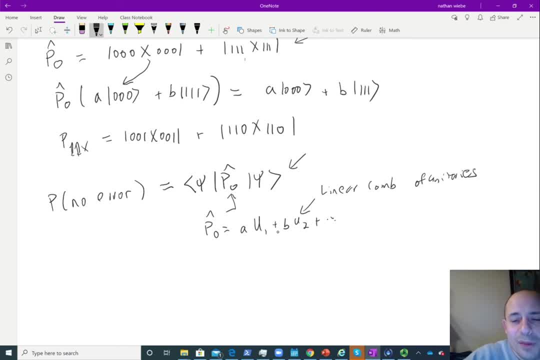 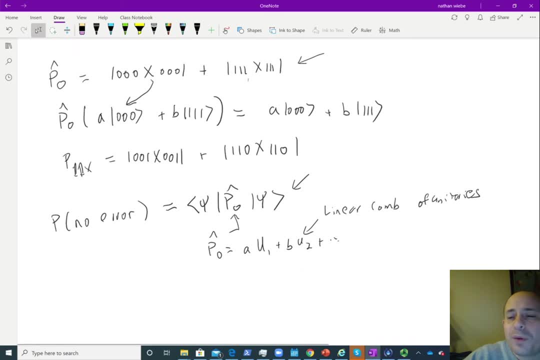 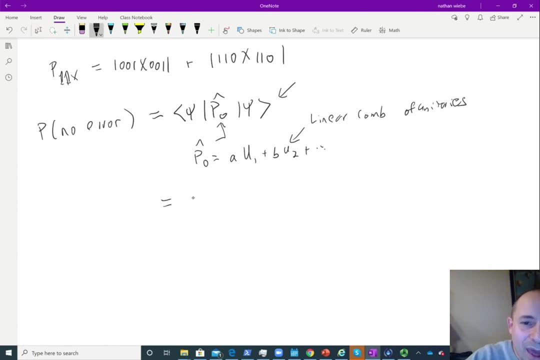 for reasons that are not totally super clear at the moment, but it will be later on when we talk about quantum simulation. but once we have a linear combination of unitaries expression like this, then we can always write this as a psi u, 1 psi plus b psi u, 2 psi plus so on and so forth. now, if we want to figure out the probability, 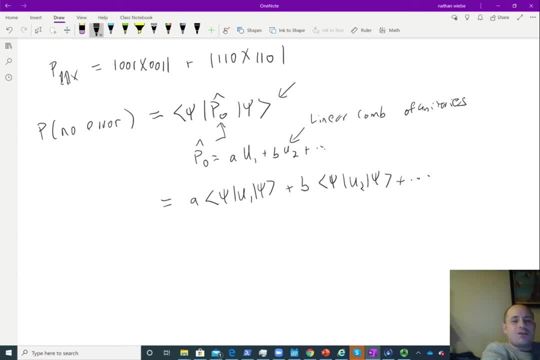 that you know we that when we measure we would end up seeing no error. we could actually estimate all of these now using a hadamard test. the hadamard test- recall- is a very simple way to do this. so if we were to take the form of the form, it looks very much like an. 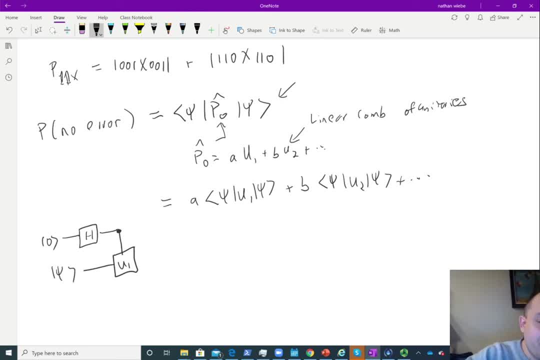 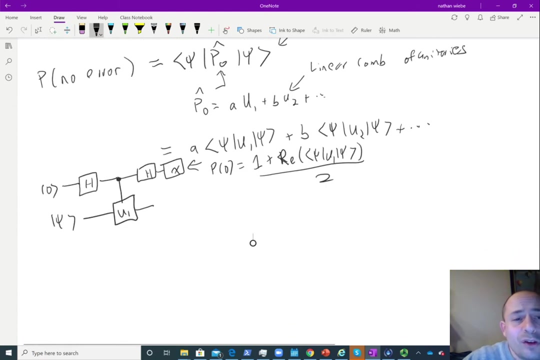 iterative phase estimation circuit. it would end up taking a form like this: psi h, and if we were to measure this bit at the top, the probability of zero is just one plus the real part of psi u1. psi over two: okay cool. so that's kind of nice, but actually we can do a little bit better. 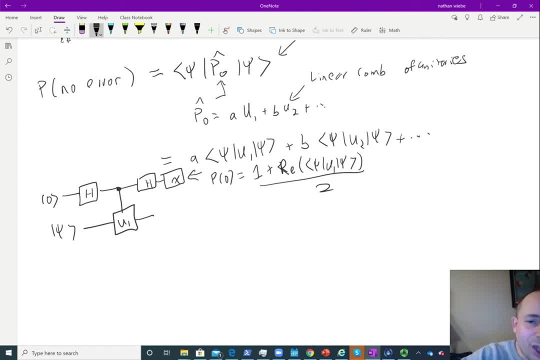 than than this. what we're going to do is we can actually further express p, not han, as sum over i, a, i, p, i, where these pi's over here? these are poly operators. so what i mean again by that is: i mean these are all operators of the form um, like i, tensor, x, tensor. 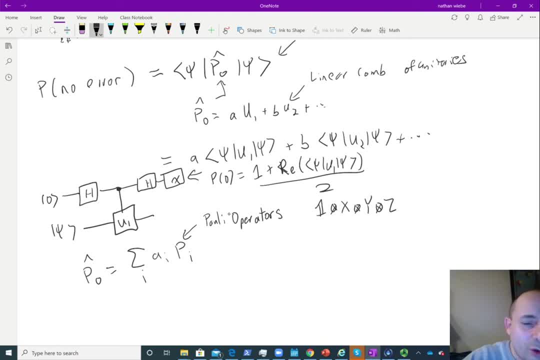 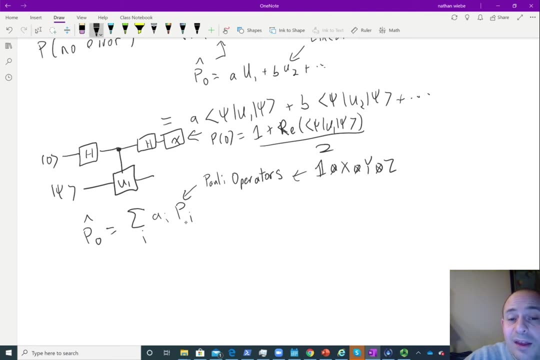 y, tensor z, so it's just a bunch of tensor products of x, y, z, and identity is what i mean by pi over here. now it turns out that one of the reasons why this is quite nice is because of the fact that all the polys are identically identifiable. 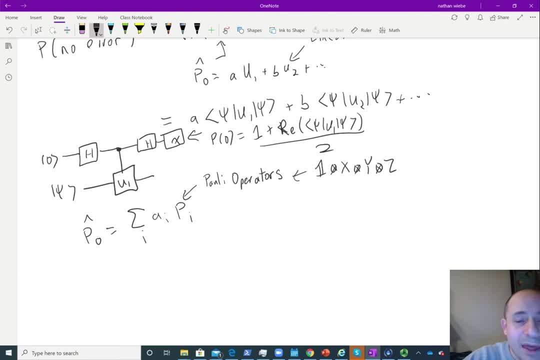 so if we look at the eigen value of some of these operators, we will find that even though they are identically identifiable, they will get a plus or minus sign. if they are in the number of the four form the order of the family, operators in this decomposition end up having eigenvalue. 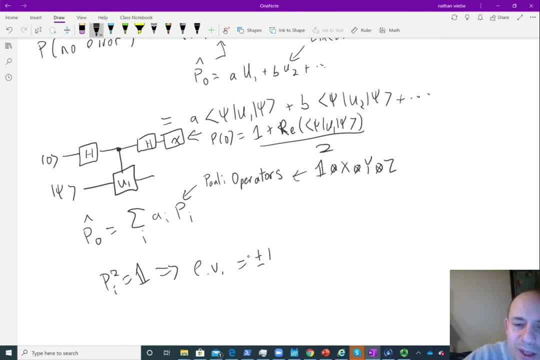 plus minus one, because p- i squared- equals identity. this implies that the eigenvalues in question are, And we can write it as psi times identity psi. Nothing's changed by that. But we can write identity as a projector onto the positive eigenvectors of pi. 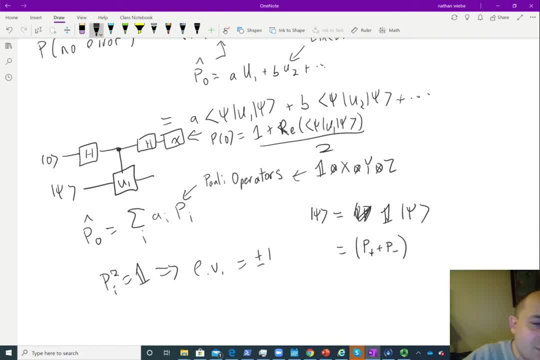 plus the projector onto the negative eigenvalues of ei. Because, basically, since every eigenvector of each of these unitaries has eigenvalue plus one or minus one, the identity operation has to be the projector onto the ones that are plus, plus the projector onto the ones that are minus, because that then covers the entire space. 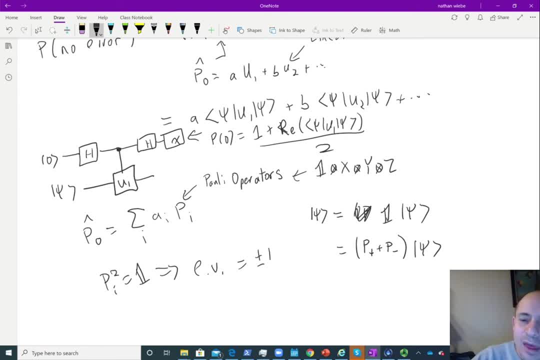 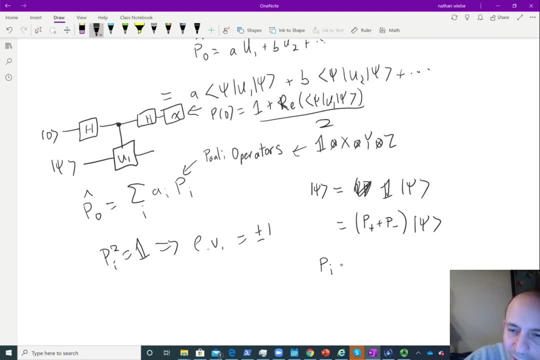 So we have the following Now: If we end up then having that pi acting on p plus psi, this by definition is just equal to p plus psi, because this is the positive plus one eigenvalues of pi. So I could also write this as just like plus one times that. 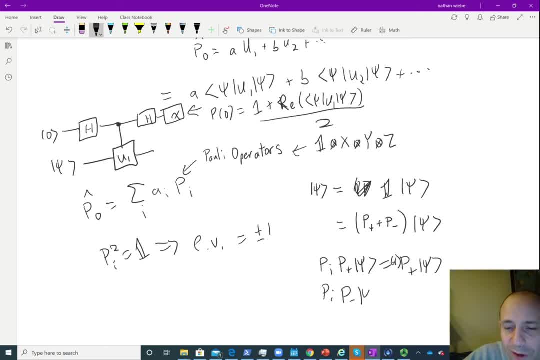 However, pi times p minus psi is equal to minus one pi, Just by the definition of the fact that p minus gives us the component of psi in the negative one eigenspace of the polyoperator. So if we end up having that, then going through the algebra for the Hadamard test over here. 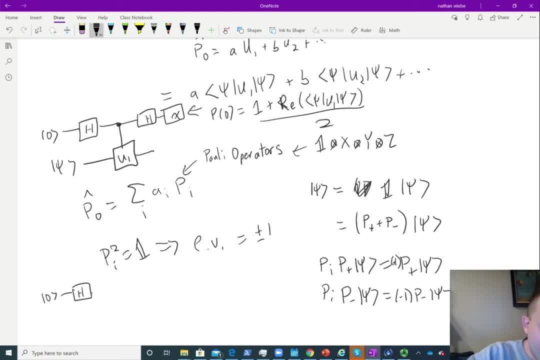 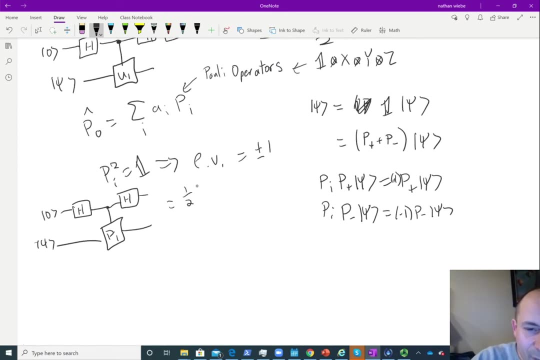 we end up getting that zero Hadamard controlled. pi Hadamard Over here for state psi ends up yielding one half I Plus, Or sorry, One half Zero I plus P I, Psi, Psi, Psi. 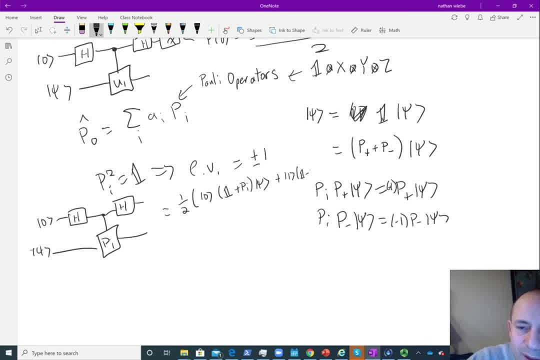 Plus One. I Minus P, I Psi. Okay, Great, Now let's. this, using the exact same reasoning, is equal to one half Zero. I Plus P. I. Now pi times p plus plus, p minus. just remembering that this is just a fancy way of me writing. 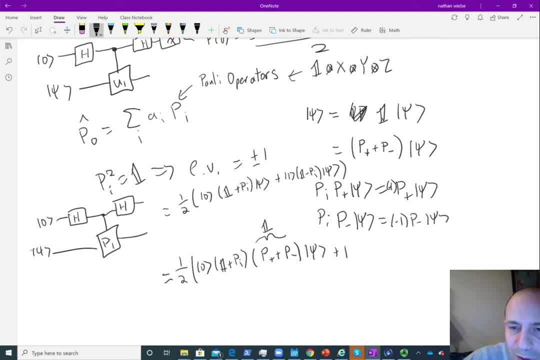 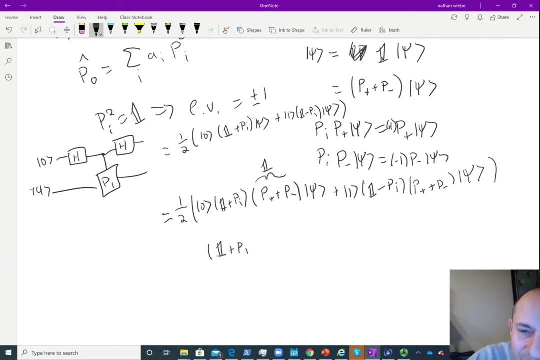 the identity matrix plus 1 times i minus p. i p plus plus p minus acting on the state psi. again, all right, cool. you might wonder why the heck did i do this? well, i did this because of the properties of p? i. let's take a look at 1 plus p i acting on p minus psi, while using these properties up here. 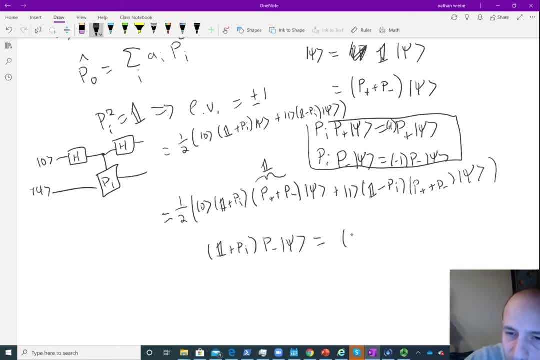 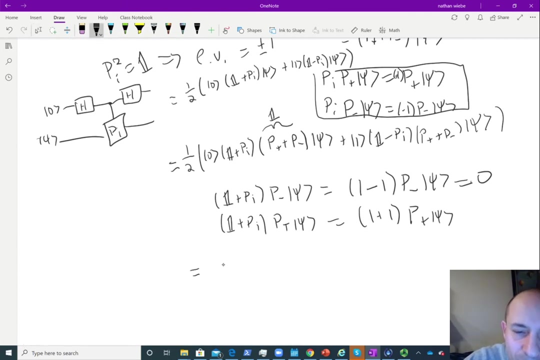 that is equal to um 1 minus 1 p minus psi equals 0. however, 1 plus p i p plus psi is equal to 1 plus 1 p plus psi. so this actually is equal to simply 0 p plus psi plus 1 p minus. 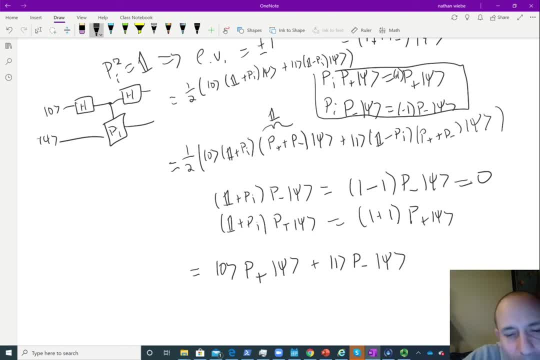 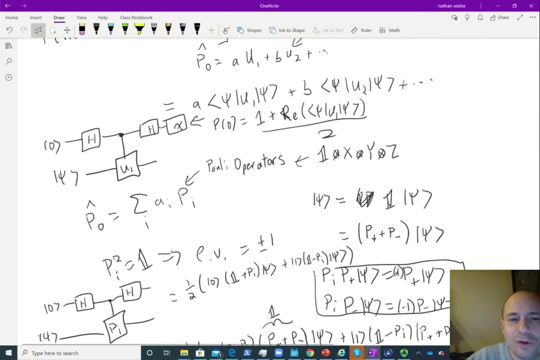 psi. so by measuring this qubit over here, we're capable of projecting our system onto either the positive eigenspace of the unit of the unitary we're measuring or the negative eigenspace of it, and we're going going to use that trick in order to be able to actually implement these projectors that we're- we're interested in. so 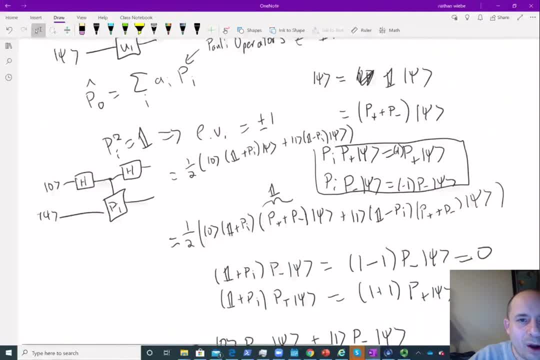 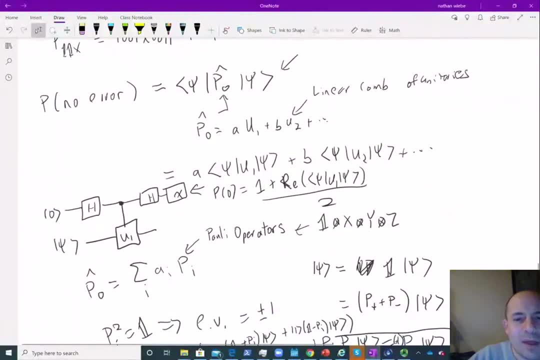 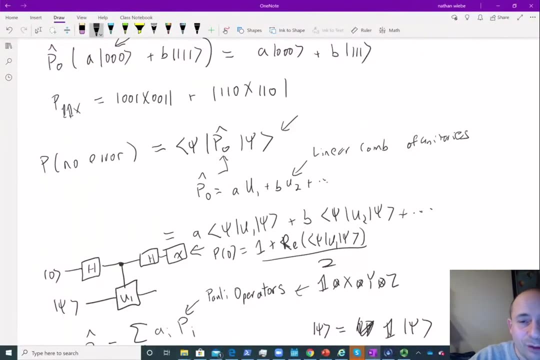 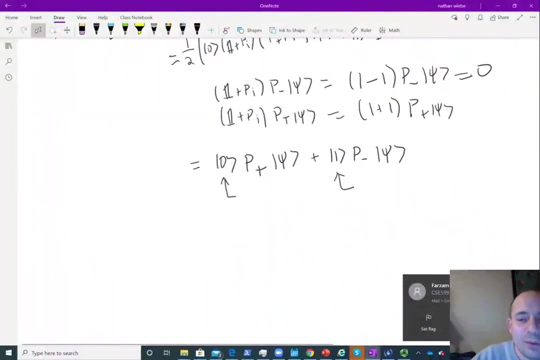 the way that we're going to do to do this is we are going to first, um, let's take a look at the poly decomposition again that i was mentioning. poly decomposition gives us a way of expressing this: no error: projector, for example, into a sequence of um poly operators that we can then deal with. so the expression let's- uh, take a look at the case. 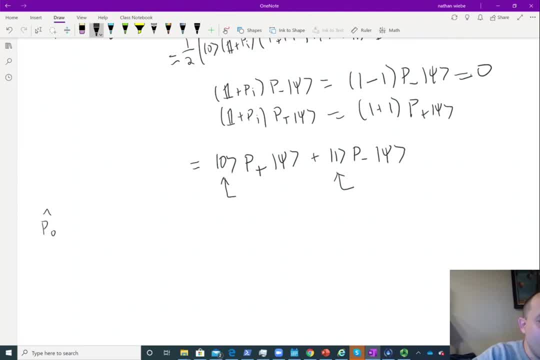 where we're doing a no error on p, not hat, is equal to um zero, zero, zero, zero, zero, zero, plus one one, one, one, one one. okay, great, now what we want to do is we want to um represent this in the poly basis, and the way that we're going to do is just again using the 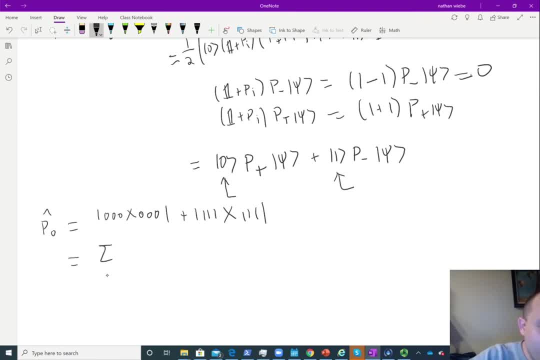 inner product form. this is equal to now. in this case, sum from i equals 1 to 63 of a i pi. now you might be worried. hey, is this guy going to go through and actually figure out all of? oh sorry, this is 0 to 63, all 64 components that we end up with. so what we're going to do is we're going to 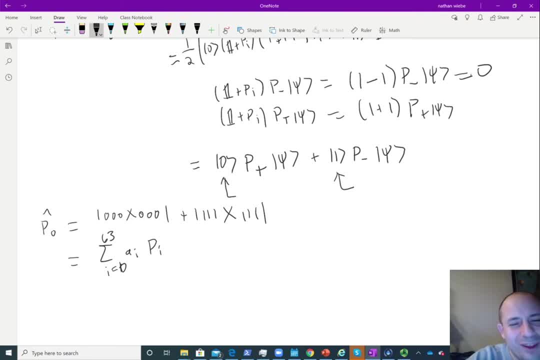 up having in here? well, the answer obviously is no, because i'm super lazy. so, um, what we're going to do instead is we're going to actually just reason about what these. these are now. the coefficients ai are, of course, given by the inner product relationship for, uh, poly operators. so, basically, 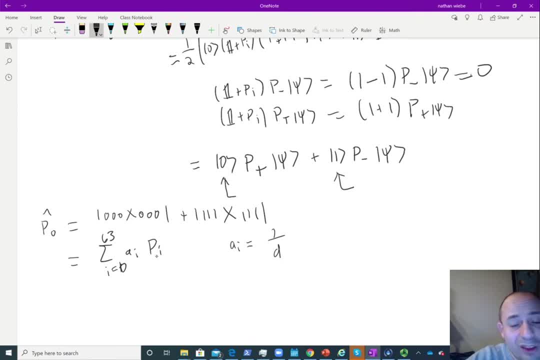 what i'm just doing is i'm using the fact that poly operators like these- pis over here- form a operator basis with respect to the trace, and so you can find this by computing the trace of the product of the projector- p p, not hat- against p i, where the trace of a matrix. 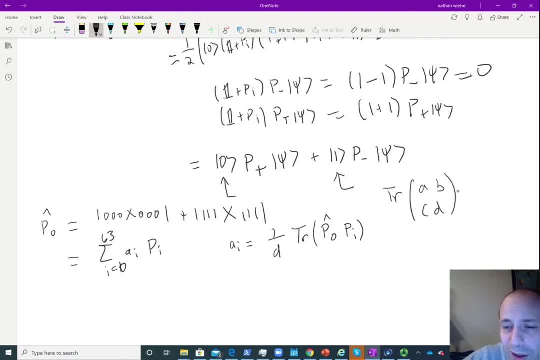 trace of, let's say, a, b, c, d. that's equal to simply a plus d, so it's just the product of the matrix and that's the, the product of the matrix and that's the. that's the matrix and that's the product of the matrix, and that's the product of the matrix. 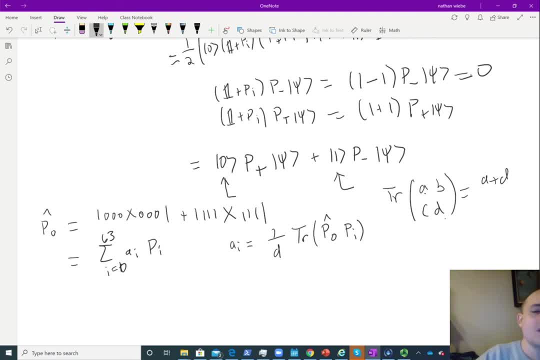 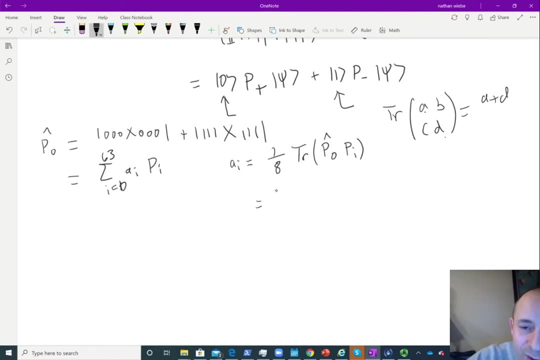 just the sum of the diagonal elements. Okay, and d- here is the dimension, in which case this is one-eighth. then, Okay, so we can see immediately that this is just one-eighth of the trace of 0, 0, 0, 0, 0 over here, pi plus trace of 1, 1, 1, 1, 1, 1, 1, pi. Okay, now there's a property. 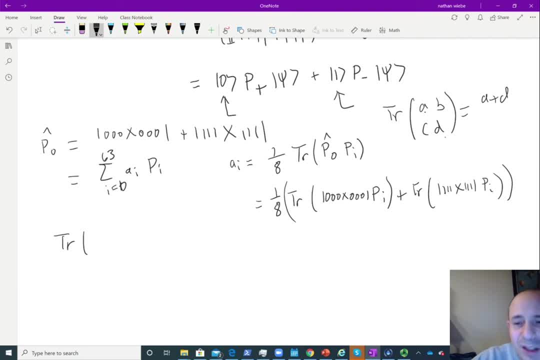 with the trace of matrices, and here I use the fact that the trace of a plus b is equal to the trace of a Plus the trace of b. This is obvious just from the definition of what the trace is, The property. that's a little less obvious is that if you have the product of two matrices, the trace of the 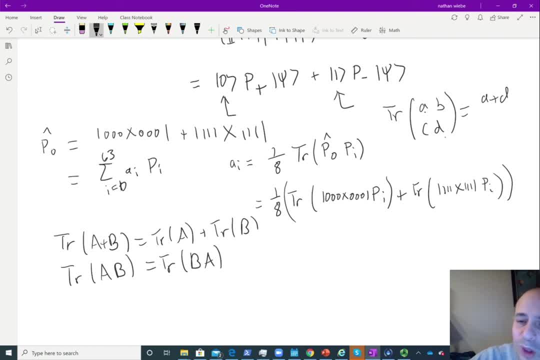 product is the trace of the product in the opposite order. So using that linear algebraic property, we can actually end up cycling this. We can end up writing this as one-half or one-eighth The trace I'm going to cyclically permute. 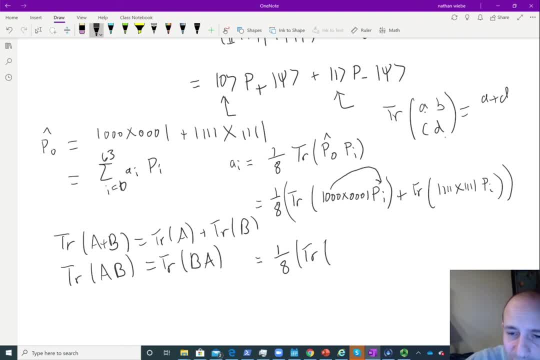 half of that projector onto the other side. So this is just 0, 0, 0, pi 0, 0, 0, plus trace of 1, 1, 1, pi 1, 1, 1.. Okay, but these are just scalars, So this is a one-by-one matrix. 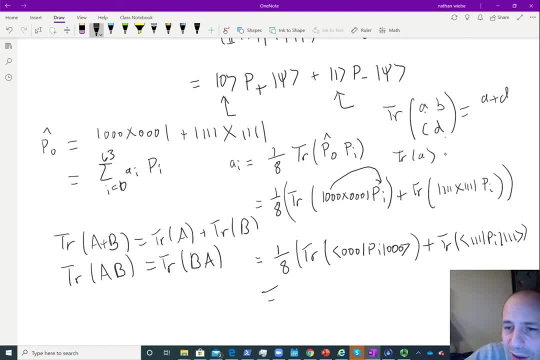 and the trace of a. if that was our entire matrix, that's just a, So we can drop the traces And this is just 0, 0, 0, pi 0, 0, 0, plus 1, 1, 1, pi 1, 1, 1.. All right, great. So now. 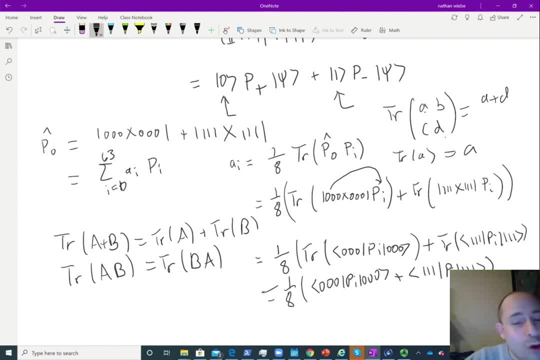 just looking at this, we can immediately rule out any component of the pi's that have an x or a y in it. The reason why is because those would end up leading to bit flips in one of these locations and thus have zero interplay. 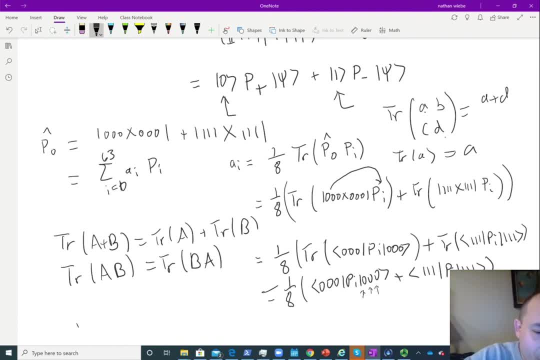 So we know that pi over here pi has to be composed of only i and z. Furthermore, just taking a look at this form over here, we can see that any term that has an odd number of poly z's is actually going to yield zero over here. The reason why is that if we have z acting, let's say we have. 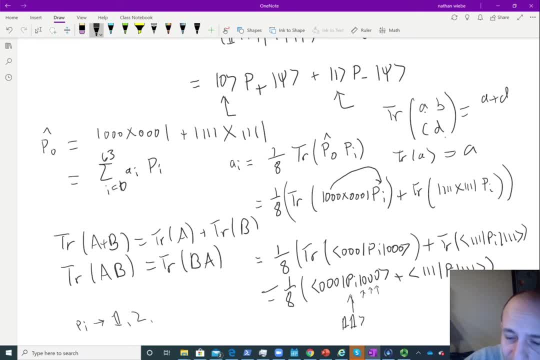 pi was i i z Well. computing this expectation value up here will end up giving us plus 1.. However, on this other side, we would end up getting plus 1 from the first one, plus 1 from the second one, because they're both identity, But the third one? 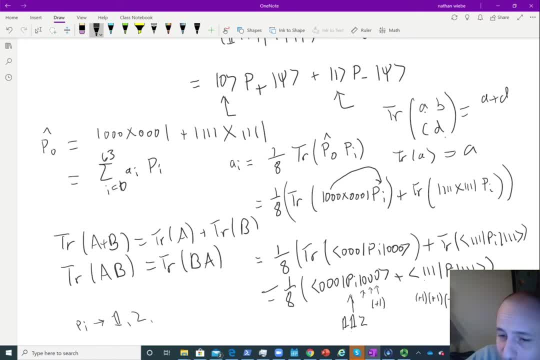 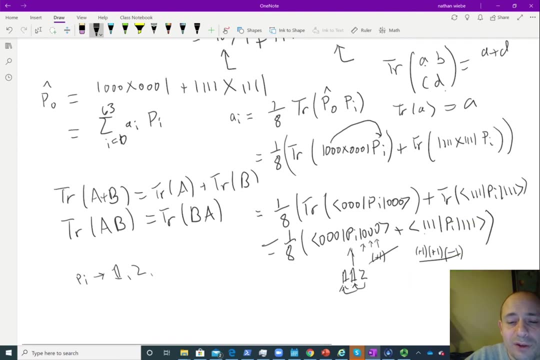 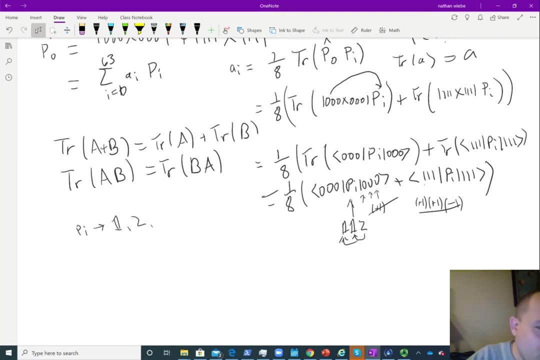 will give us minus 1.. So these two are going to cancel, giving us zero. Therefore, the only ones that remain are the possibilities with two or zero z's, And so we can end up seeing, actually, that this ends up taking a form one quarter identity plus. 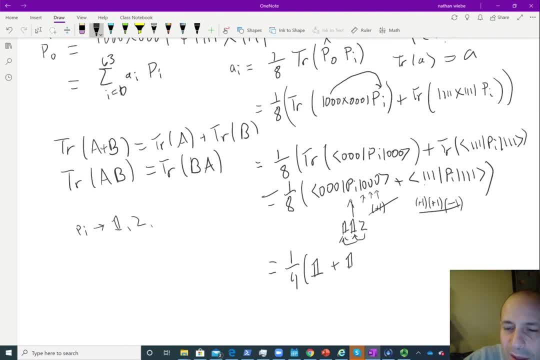 this one. So this identity is z z plus z i, z plus z z i. This identity term doesn't matter for our purposes. The things that we need to take a look at are these. So now what we can do is we can project onto p0,. if we can project onto p0,, we can project. 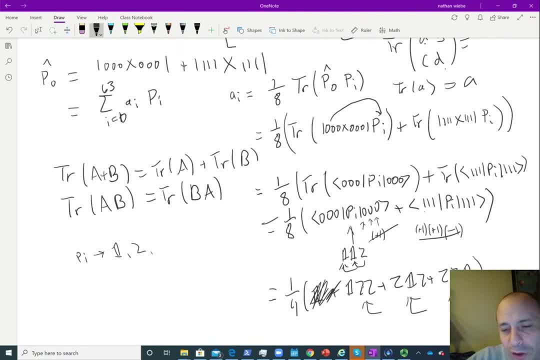 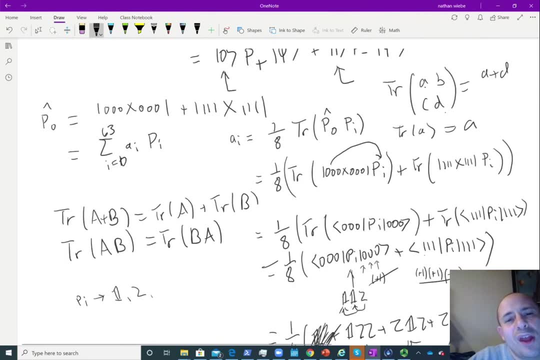 onto the superior value quater. Now let's start with, in general, máxim Fitness. So, for examples, this would be gundam. So let's identify two of the derivatives into one like this, And then we would project onto ZZ, ZIZ and ZZ, And the way that we do this is by using a Hadamard test in order to 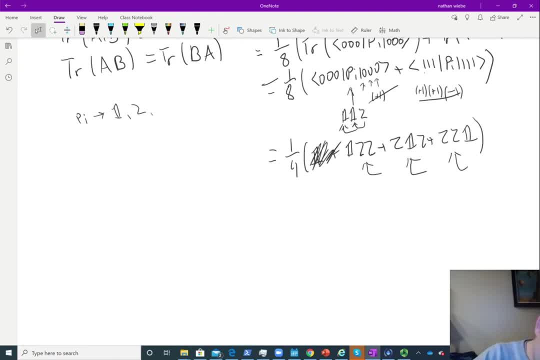 try to project onto the plus one eigenspaces of all of these. So way we do, that is as follows: We take our input state psi over here, We do the Hadamard test in a piecewise fashion- Oh whoops, sorry. We begin with psi over here and we compute. 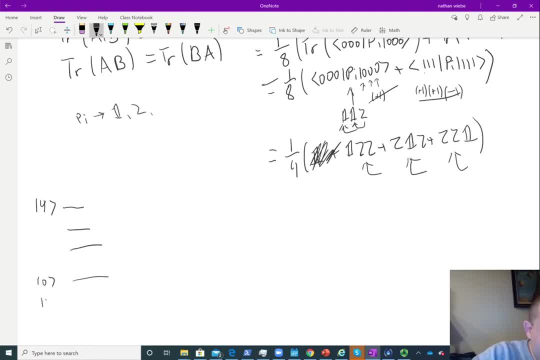 the Hadamard test by preparing three extra bits off to the side. We apply Hadamard transforms here, And then what we do is we just go through this pattern. So first I'm going to apply two ZZs here, Okay. Next, what we're going to do is we're 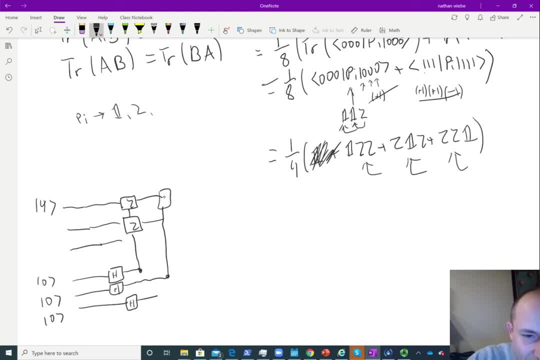 going to do the next one, which is ZIZ, So I'll project onto that And oh, whoops, here, Nope, There, Yeah, And then finally I'm going to go here, here and not there, Okay. 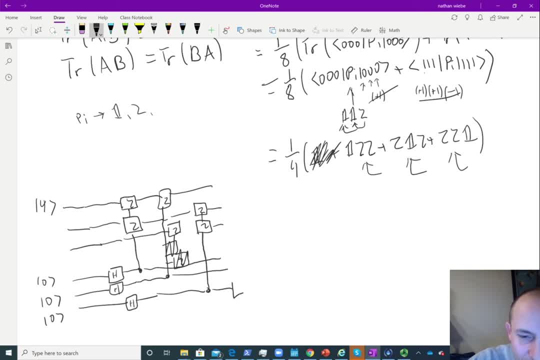 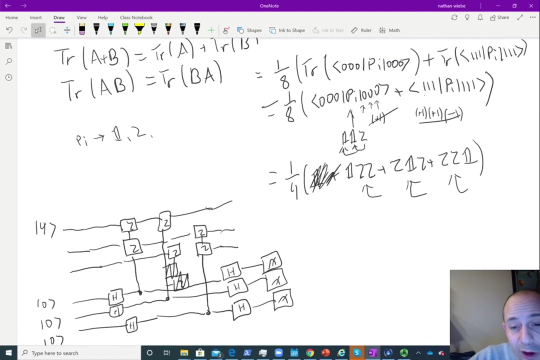 Yeah, And these guys fly through And as a result Is I try to triple-ц- all these same walk melt in together. So okay, Now I Hadamard, Hadamard, Hadamard, and I measure. 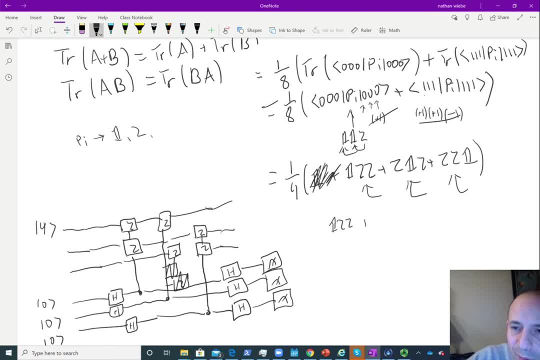 Okay, In the event that I project onto the plus one eigenspace of each of these, That corresponds to applying IZZ plus ZI ukw I, ZR z plus z z i and that is equal up to an identity to p, not hat. so in the event, 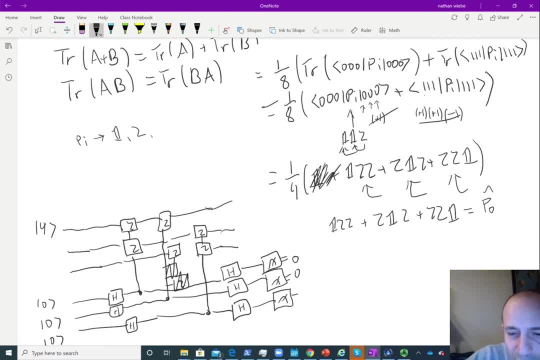 that all of these guys come back measuring zero. that corresponds to no error- and then you rejoice. however, in the event that one of these comes back as one- let's say the third one comes back as one, then what we've done is we projected on to the plus one eigenspace of this one, plus one eigenspace that one. 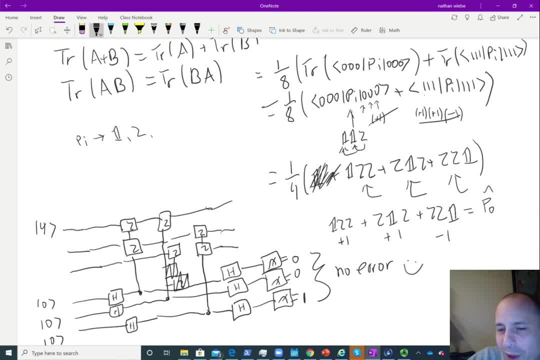 but the minus one eigenspace of this one, meaning that in this case, the first two or the last two are correct, so these two are consistent. these two are consistent. however, these two are not, so this corresponds to a, to a single error that we can then track back using using the similar orthogonality. 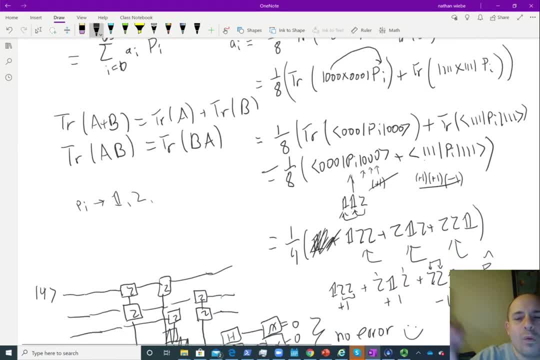 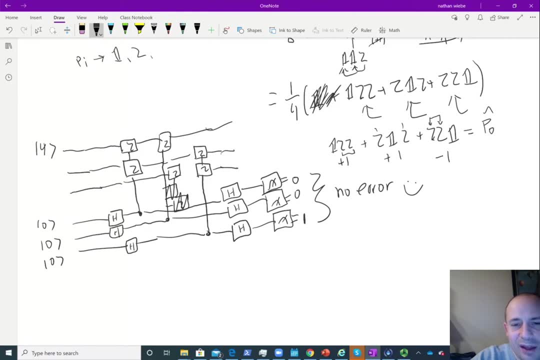 equation, example, considerations and figure out what error we exactly are going to have, and then we apply where we apply, corresponding x-gate- I think it's to this one over here and conditioned on that. so this is the syndrome extraction, and the final step that I discussed involves the correction, and this is how we can end up. 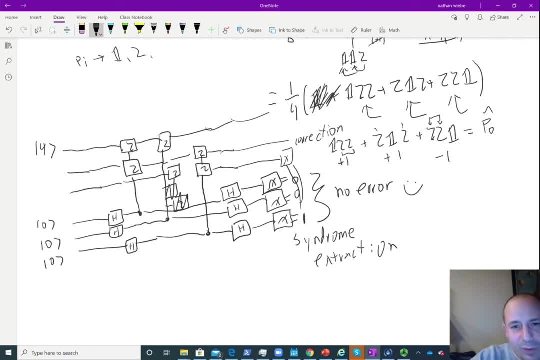 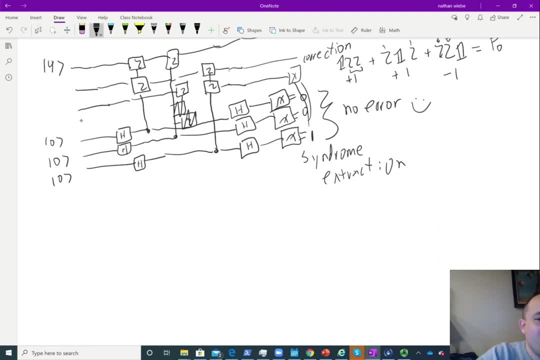 doing quantum error correction for the bit flip. okay, and if we wanted to do this with even more redundancy, we could just simply repeat this with a couple more lines, in which case we would- we would just simply have more patterns to end up going through in order to be able to infer this: what errors did happen? 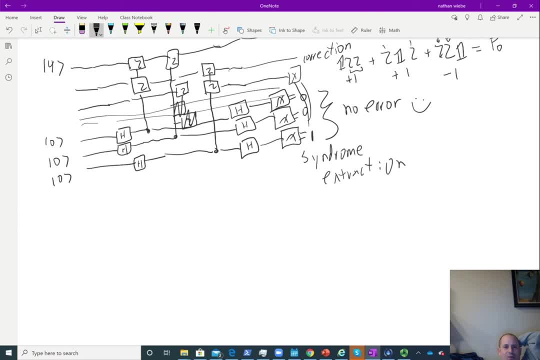 based on all of these Zed measurements. so the biggest weakness about this is that it clearly, clearly cannot deal with every type of error that we could conceivably have in the system. for example, let's say that what we have is we have the a 0, 0, 0. 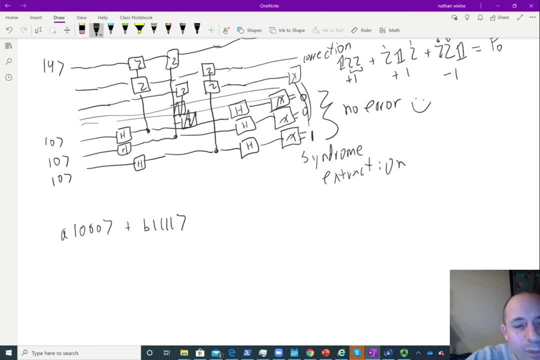 plus B 1 1, 1. now, if I end up, instead of applying an x-gate on the third bit, I applied a Z gate on the third bit, then this would end up mapping us to a 0 0 0 minus B 1 1, 1. okay, now we would send this through all. 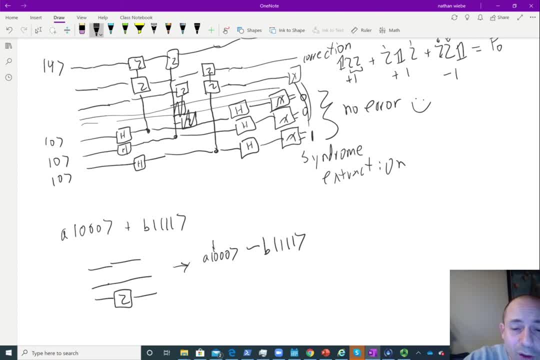 of this over here, we note, because all of these bits haven't flipped over here- we would end up getting actually all three of these being zero, and this would go through the quantum error correction phase and literally be decoded as that state over there. and this state is not correct. the sign: 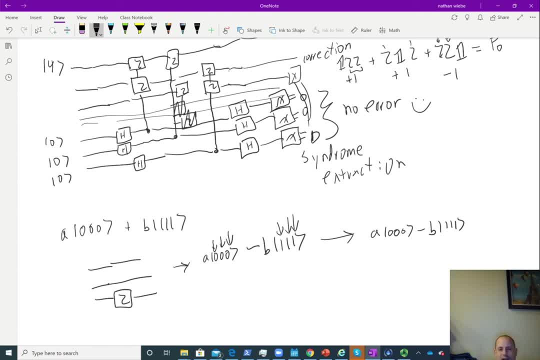 on the uh. the second code word, the logical one, is opposite of what it should be. so what that means is that means we've got a major problem, that there are physically important errors that just simply having a bit correction, bit flip correction will not be able to address, and this is something that 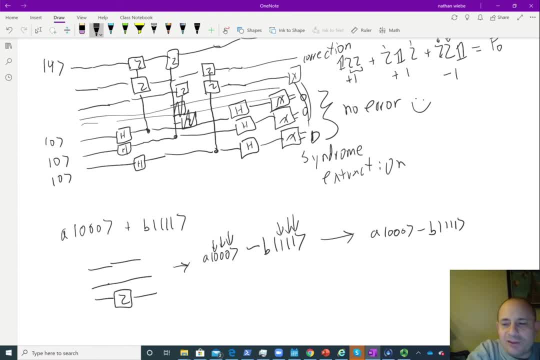 is unique to quantum and we'll see next lecture a technique for dealing with this and the idea basically is that what we can do is by using Hadamard transforms, we can convert this phase flip into a bit flip, So we could also come up with a quantum error correcting code to be able to deal with the phase flips. 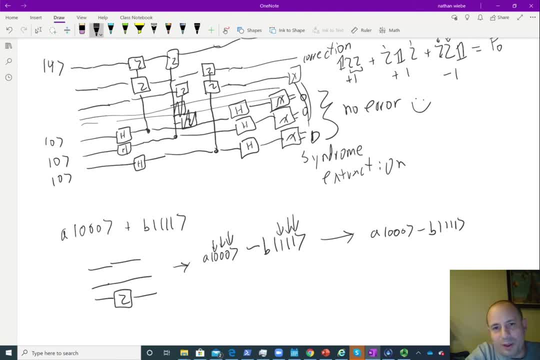 But if we did so we would lose the ability to correct the bit flips. But by concatenating the two codes, one on top of each other, it's actually possible to create a nine bit code that's capable of tolerating both a bit flip and a phase flip.